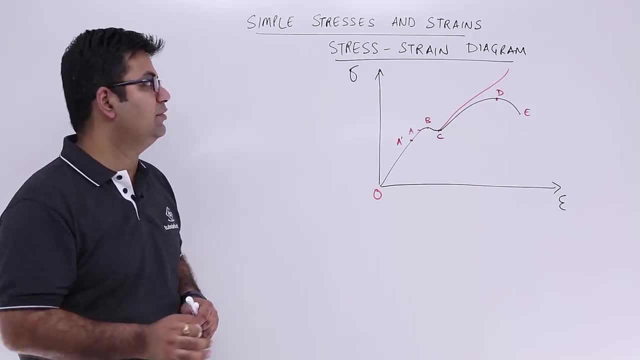 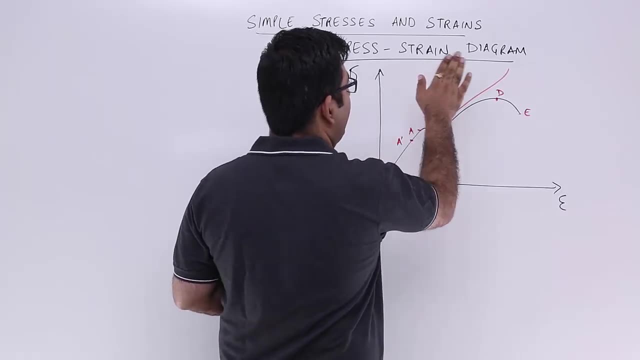 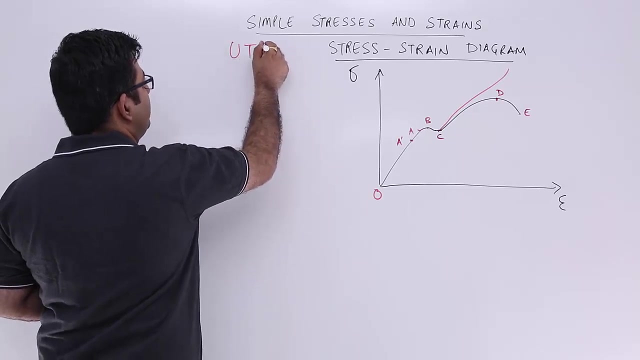 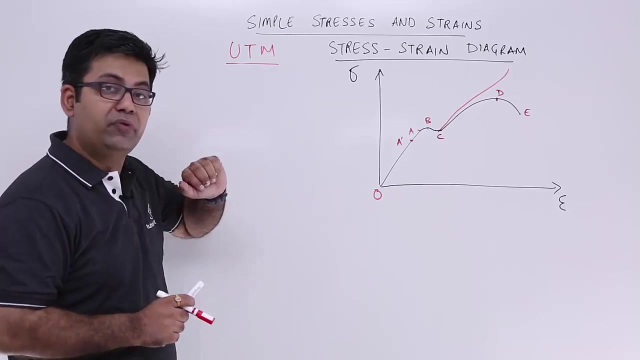 Now let's apply the knowledge of stress, strain and elastic limit onto this diagram. This is what we call a stress-strain diagram. This is a diagram which is drawn with the help of a universal testing machine, that is, a UTM. We are not going into too much details as to how do we achieve this kind of a graph. We are going to analyze this graph. 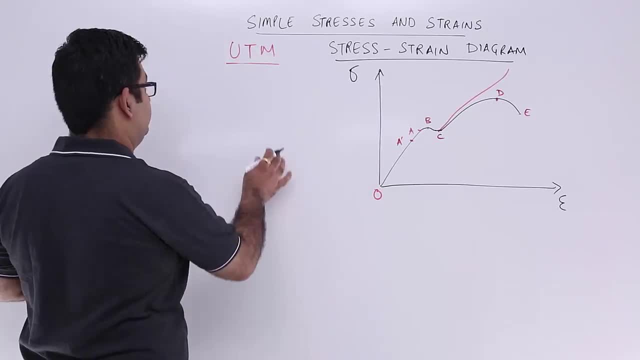 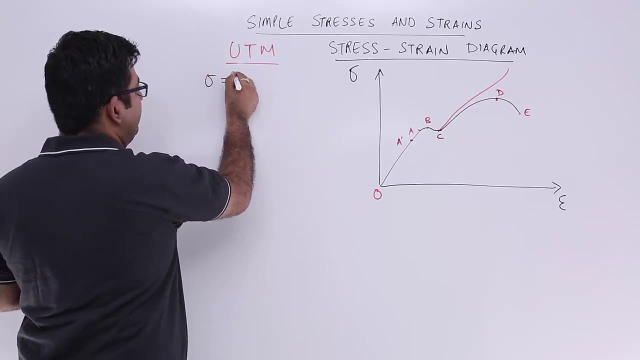 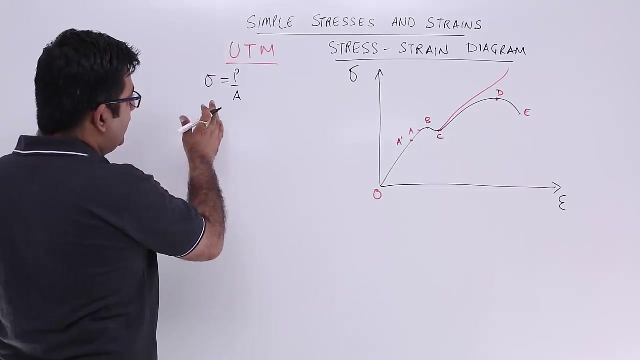 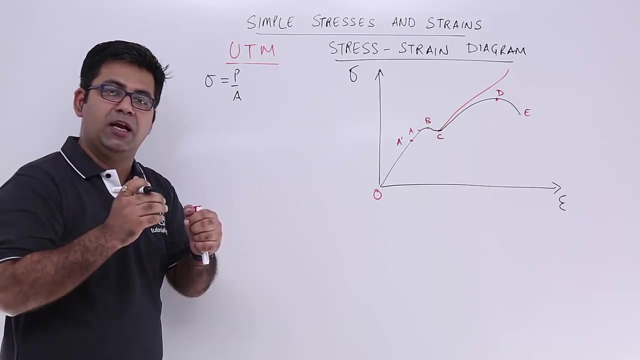 Now there are two kinds of stresses basically. So I told you that sigma is equal to load upon area. Now, if you keep on pulling the body, it will keep on getting thin, The length will keep on increasing, But the cross section area will keep on increasing. 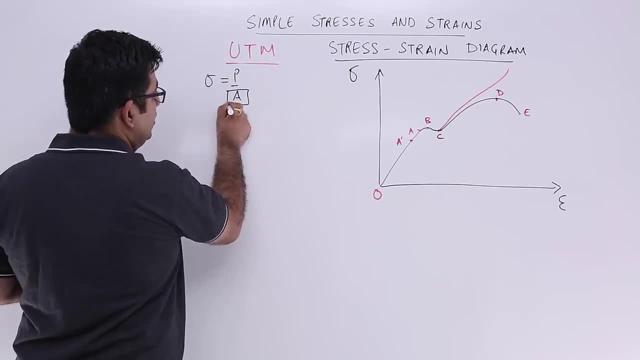 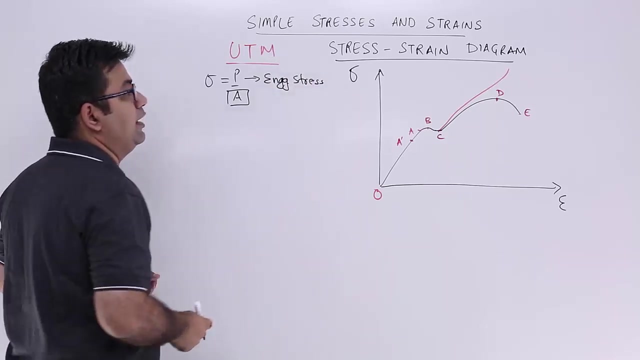 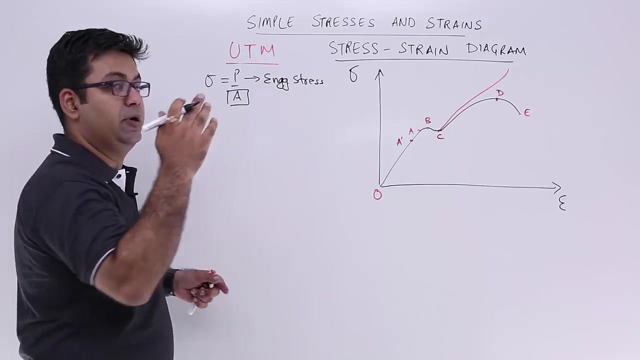 But over here we assume that the area remains same throughout. So when we assume that that kind of a stress is called an engineering stress, Because this is for engineering calculation purposes only And the corresponding strain is called engineering strain- On the other hand, if I talk about 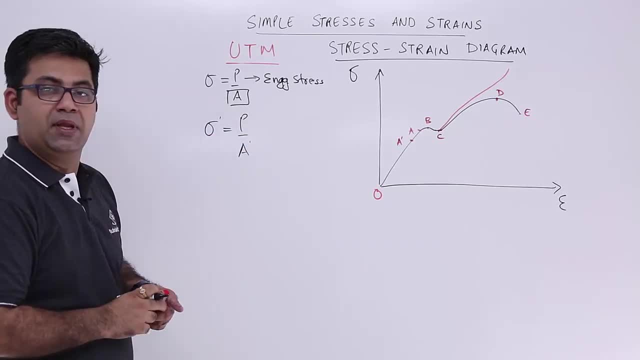 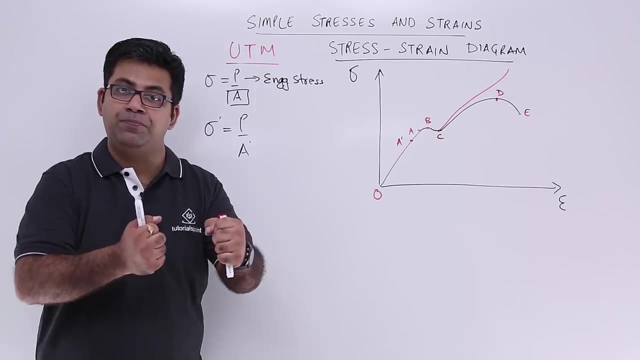 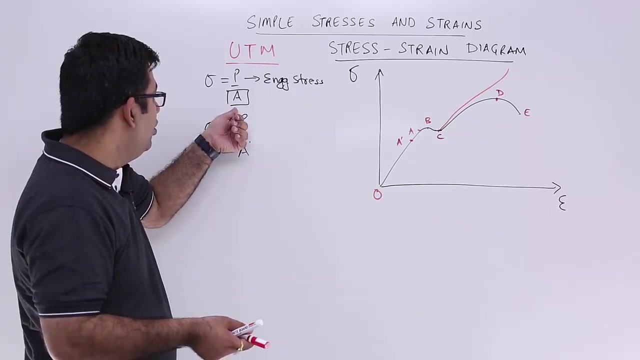 This Dash Dash means instantaneous area, Because at each increment in the length you will have a decrement in the area. So your stress value will be different at every load and at every area. So you have both the things changing Over here. area is constant. 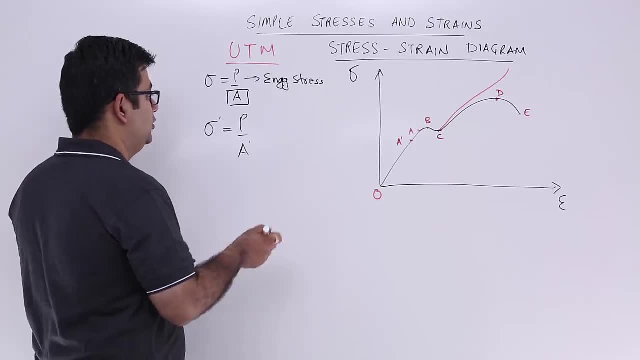 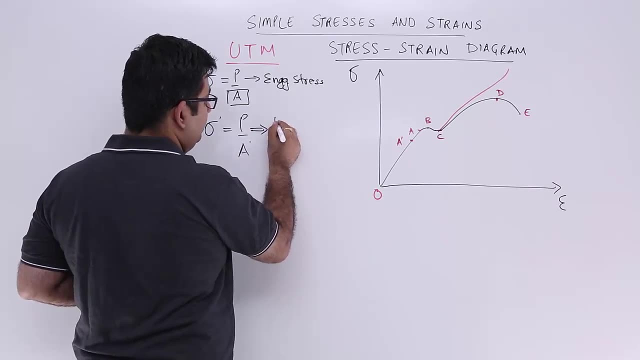 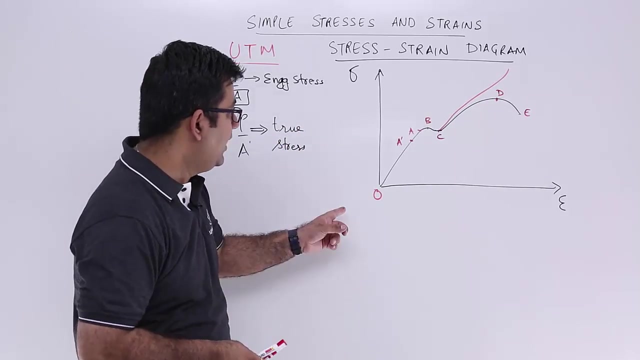 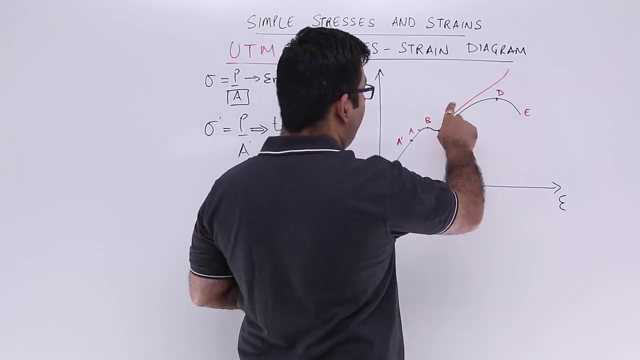 But over here the area keeps on reducing. So this kind of a stress, which is correct, Which is corresponding to the instantaneous value of area, is called true stress. And you can see that this black colored graph is representing the engineering stress And this line, this red colored line, 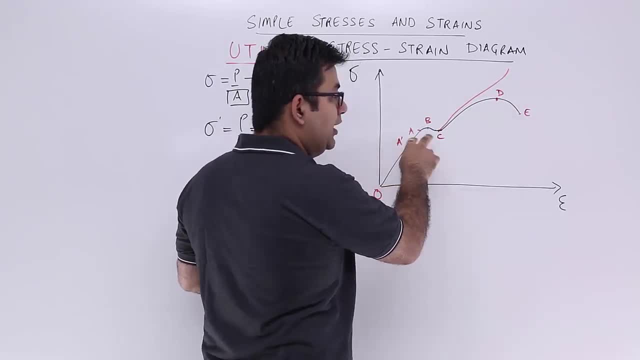 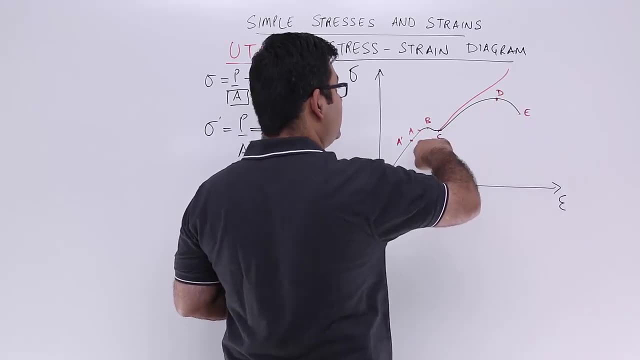 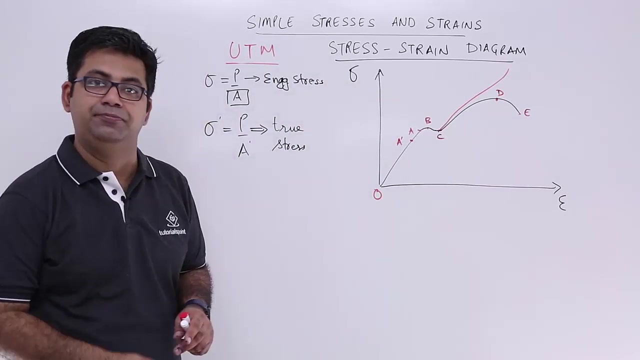 So this black colored line up till C is almost same for engineering stress and for true stress, But From point C This red colored line Is indicating the true nature of this diagram. It means it is depicting the true value of stress. Okay, 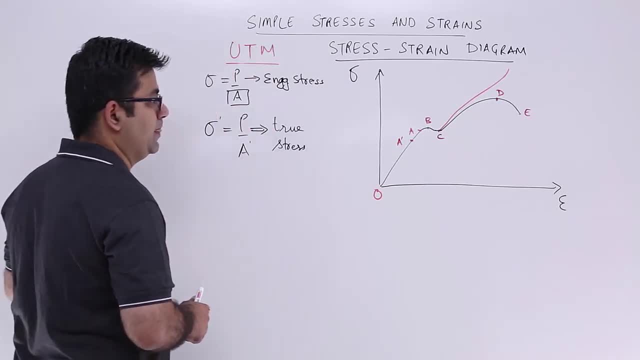 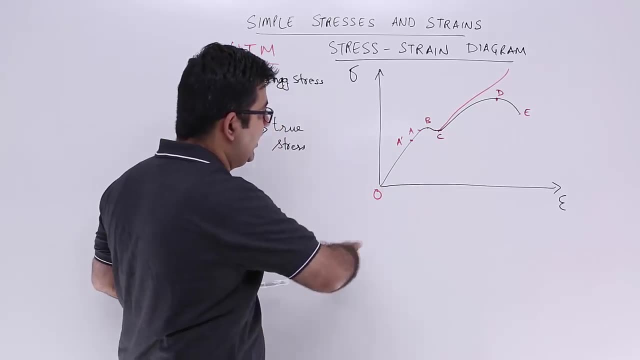 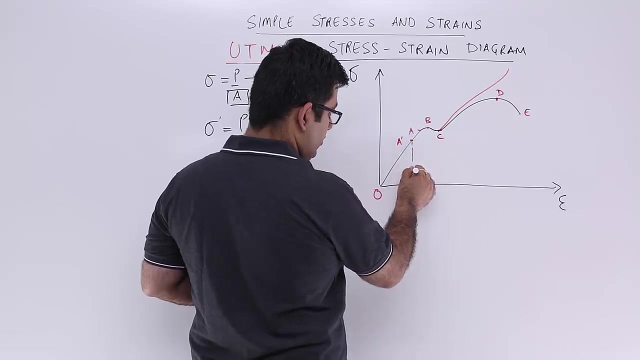 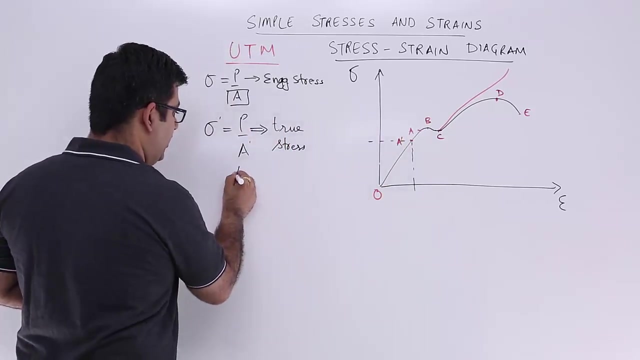 So let's Annotate these points. So, Up till From point O to A dash, You can see that the behavior is entirely linear, Okay, So If you Mark this point, This point A dash over, here Is the proportionality limit. 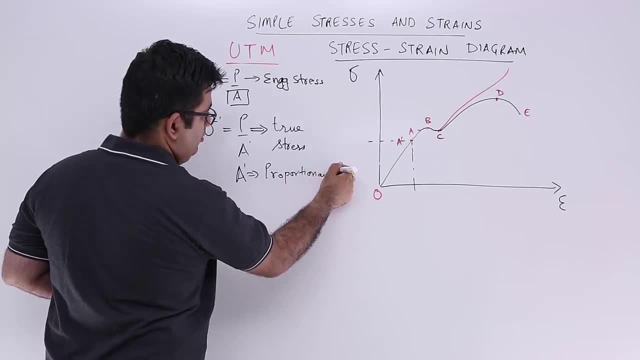 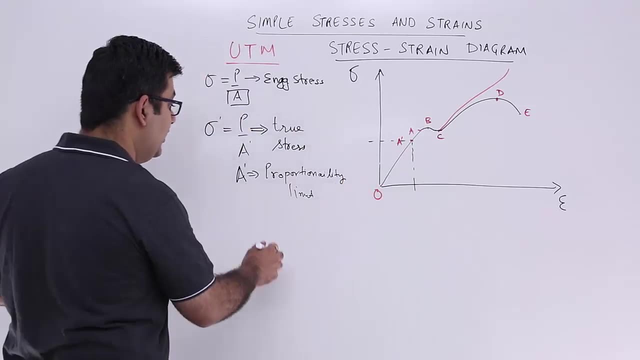 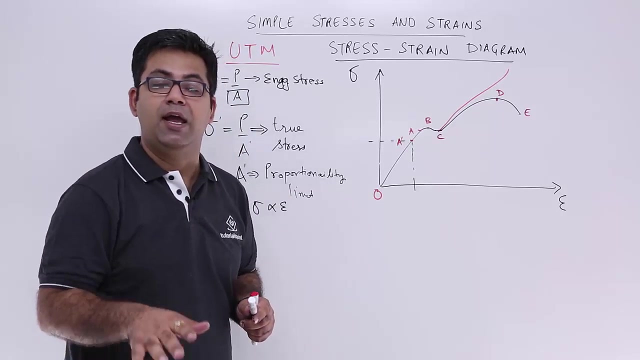 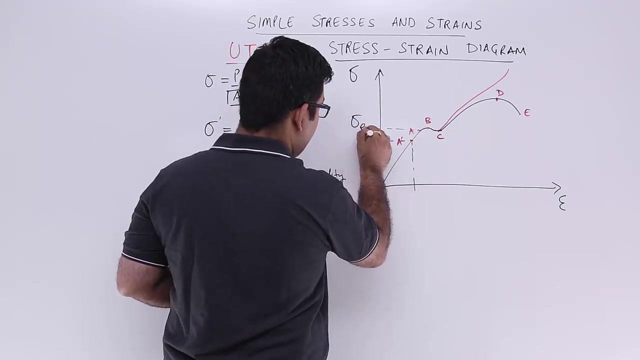 Proportionality Limit. By this we mean That up till point A, Up till point A, Stress remains proportional to strain, But It is not the elastic limit. In reality, Elastic limit Is at point A, So this is the elastic limit: stress. 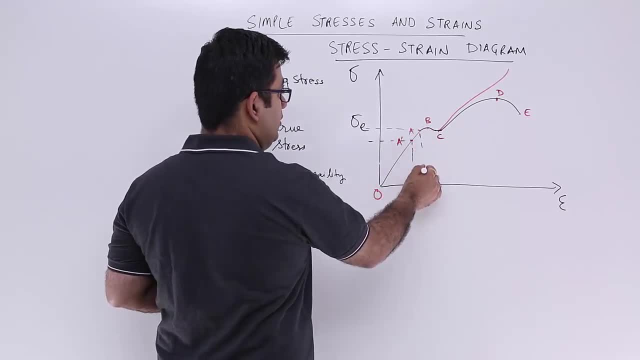 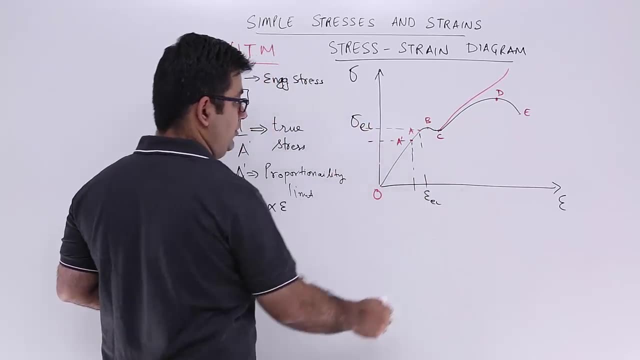 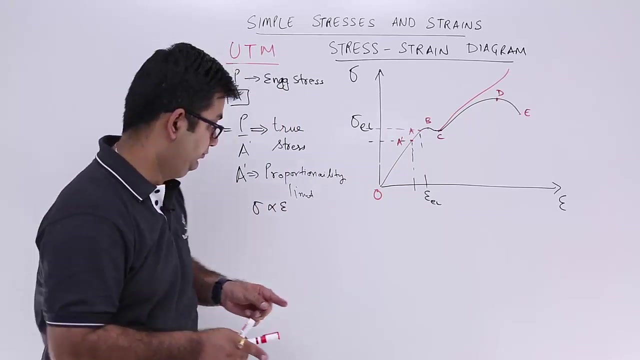 Sigma E, The corresponding strain Is called Epsilon E, Or I can say E L. Okay, So At point A Your elasticity will finish off. But The relationship Between sigma and epsilon Would not be entirely Linear. 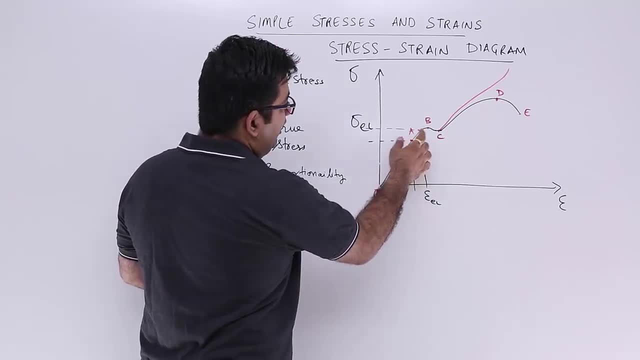 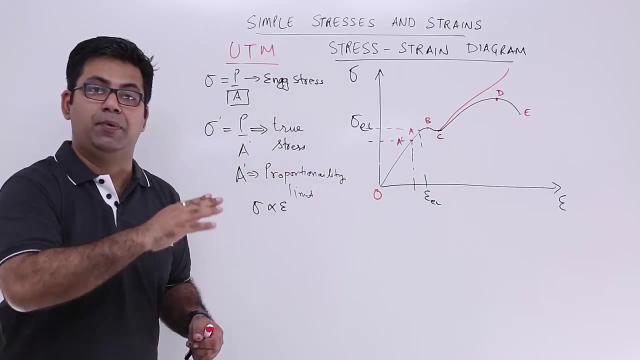 It will be little bit curved, But this gap Is not that considerable. Okay, So This is a very, very short line, But it is not entirely straight. The proportionality Is only up till point, A dash, Okay. So if you draw this, 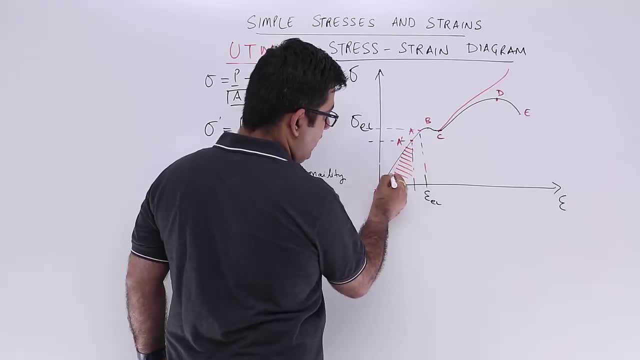 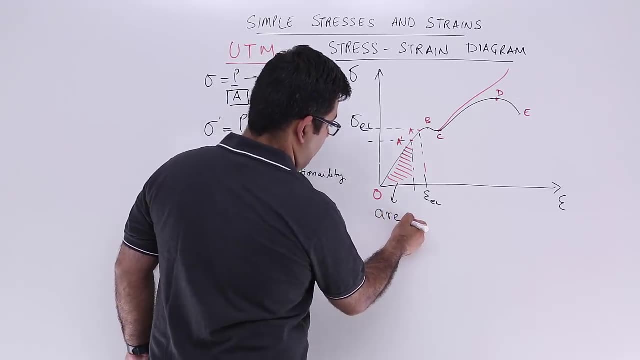 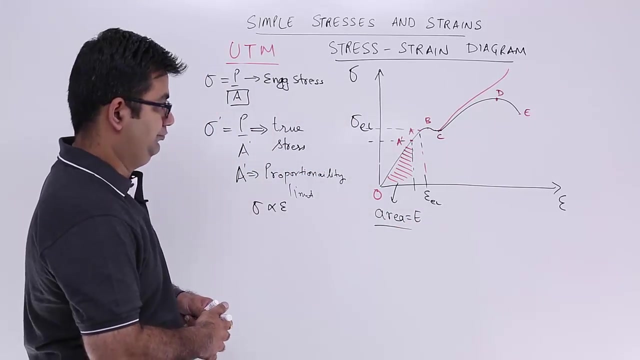 Line over here, This area, This area over here, This is called Young's modulus. This area, It represents The value of Young's modulus. Okay, Now, If you move ahead, If you go beyond The elastic limit point, 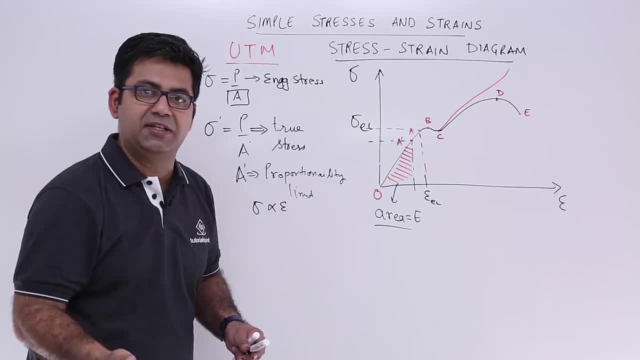 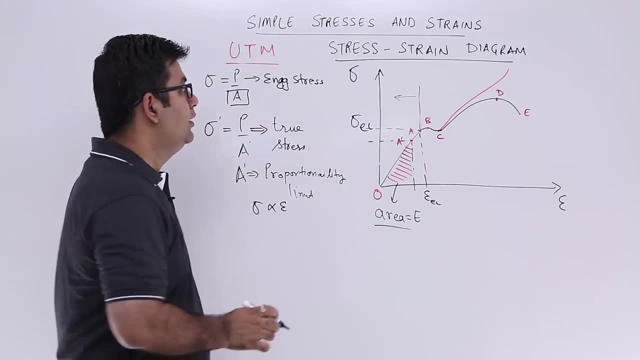 If you go beyond this point, So Towards the left of this line, You are Entirely In the elastic range. If you remove the load At this point, The strain would become zero. But If You move Beyond, 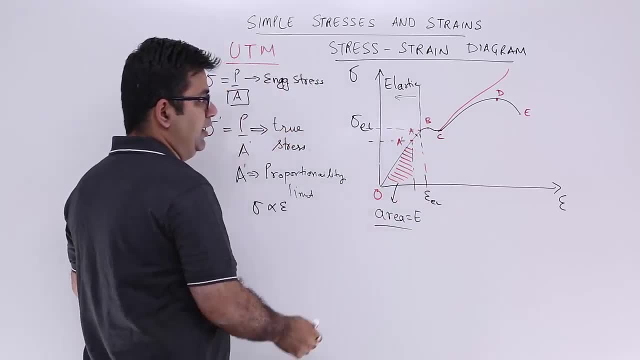 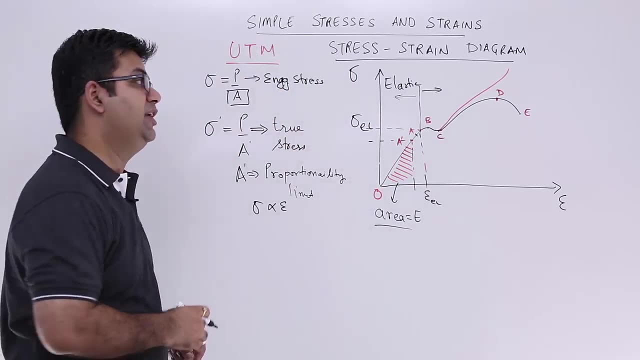 This line Or this point, You are Entirely In the elastic range. If you remove the load At this point, The strain would become zero. But This line Or this point A, You come Into the plastic region. 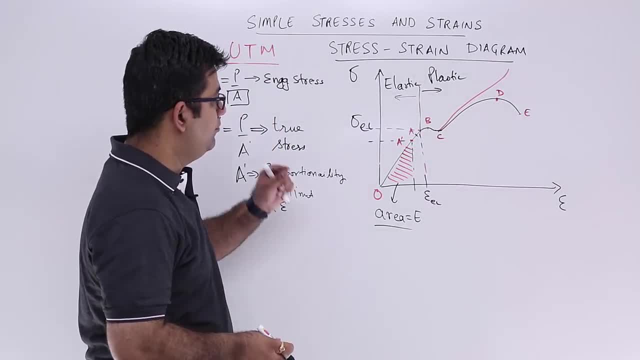 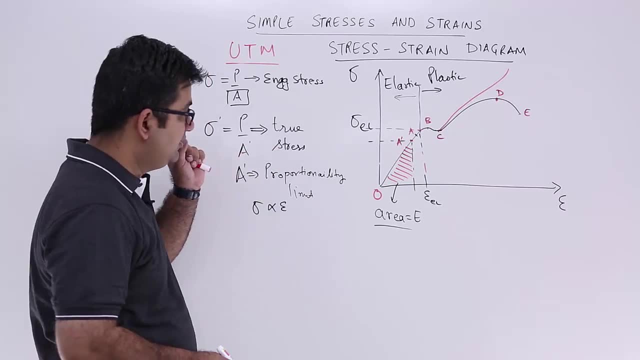 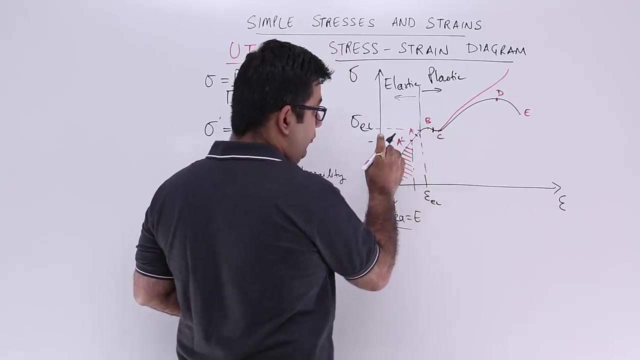 That is, Upon Removal Of the load, You will not see, As You know, Hundred percent Reduction In the Strain. You will Still, Still see Some amount Of deformation There. So Let us say: 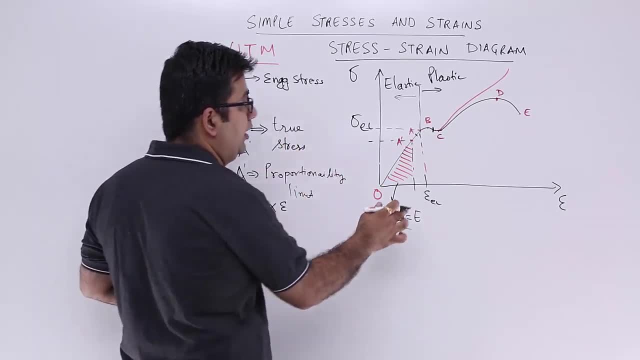 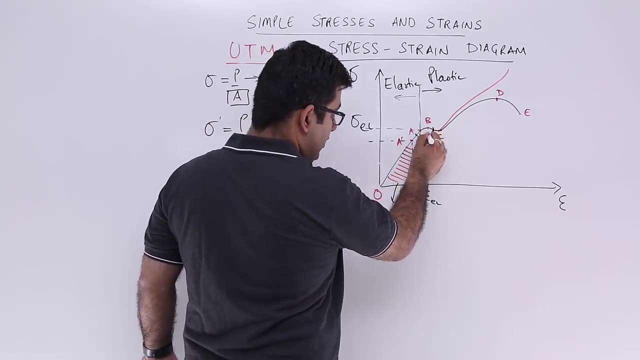 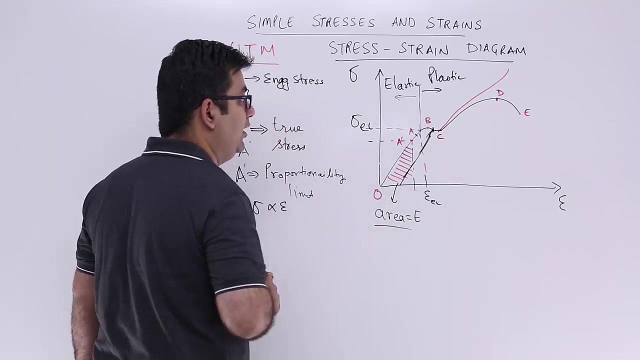 You are at point. This is the point. I am not Right now Describing points. So When You remove The load, At that Point The Strain Falls Like This: Okay, This. 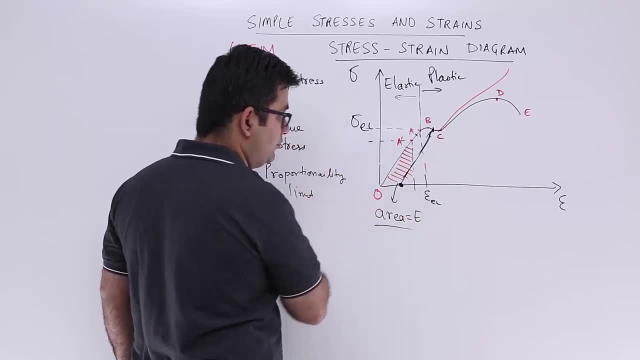 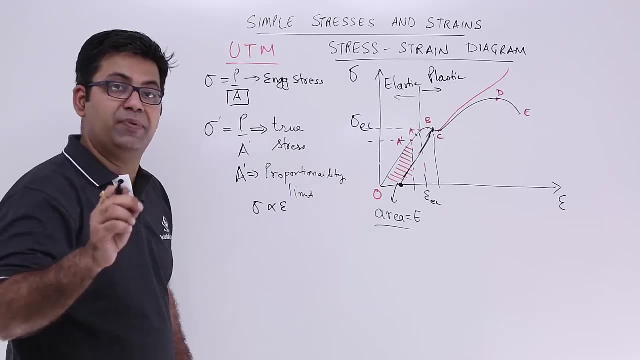 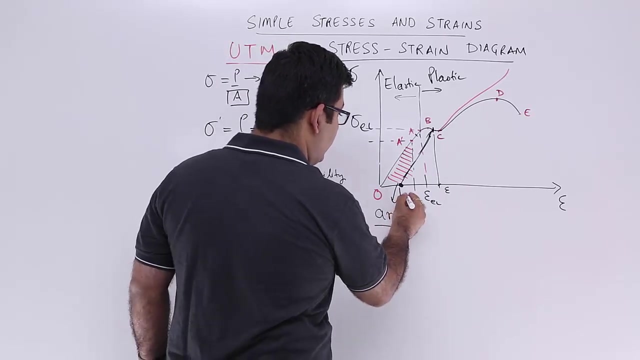 Is How The Strain Will Decrease. So You Still Have Some Value Of Strain Initially. This Load, This Much Strain Vanishes Off It. 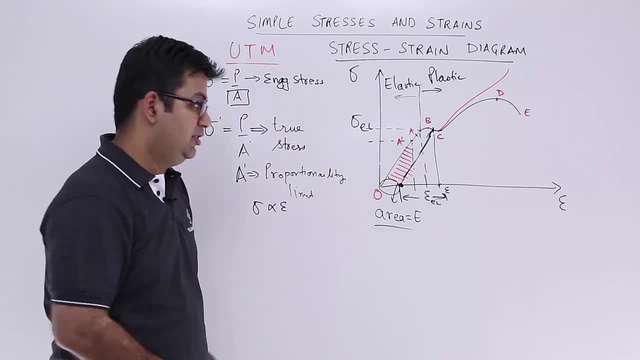 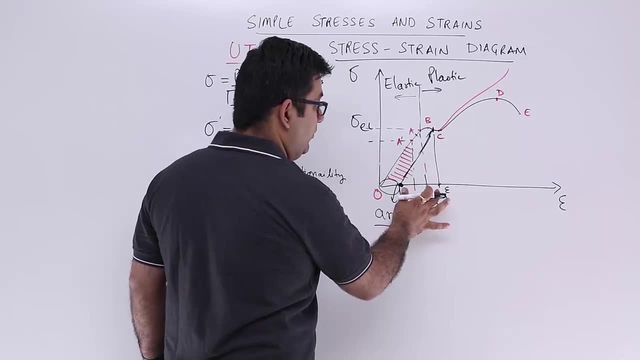 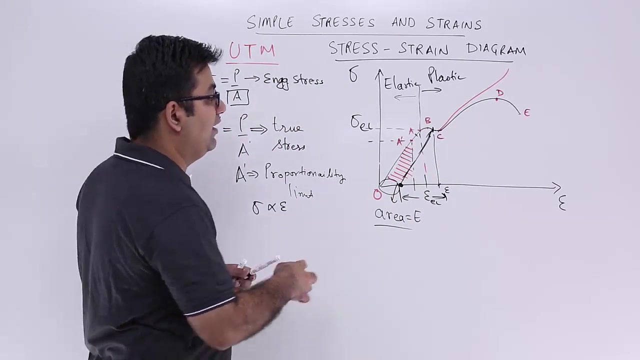 Is Nowhere To Be Seen, Okay, But This Much Strain Is Still There. So This Is Called The Permanent Deformation. That Has A Point. 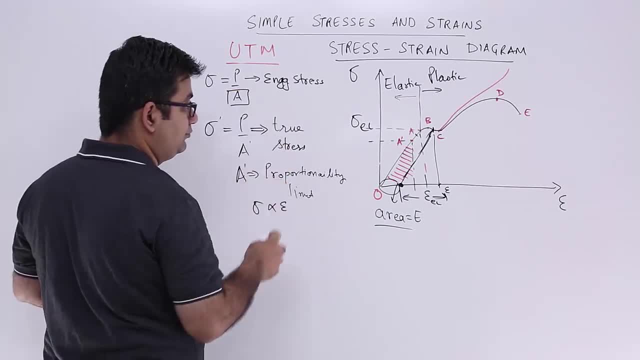 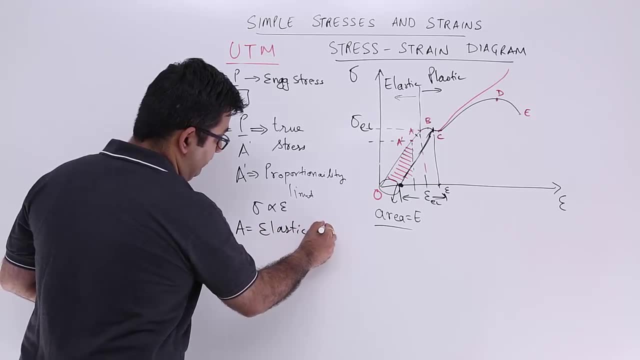 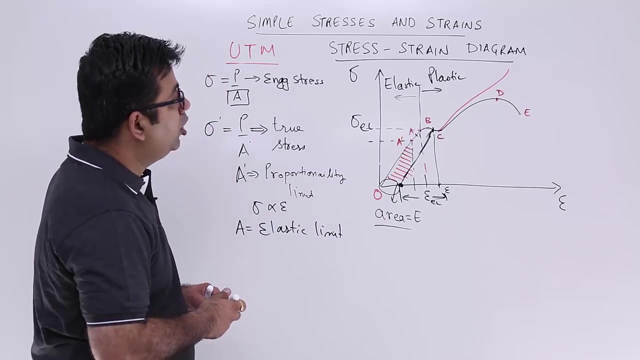 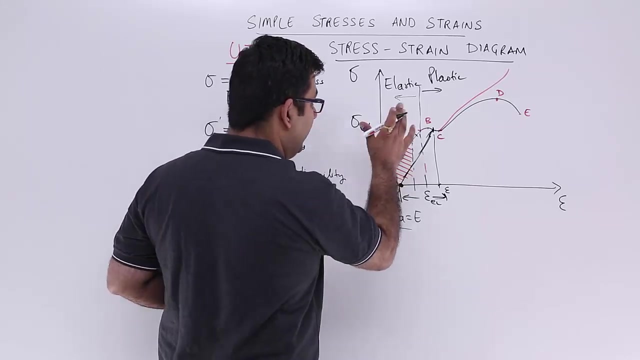 A Dash, Which Is The Proportionality Limit. Point A, Point A As The Elastic Limit. It Is The Point Up Till Which The Material Behaves. 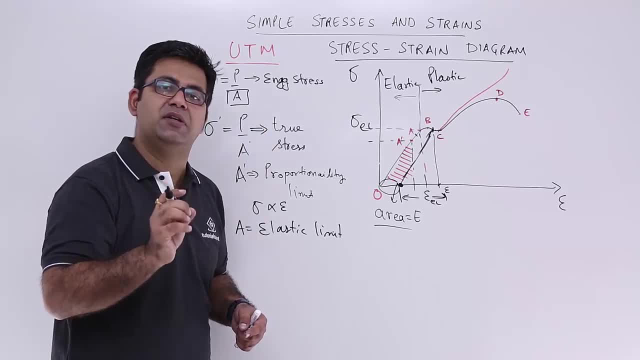 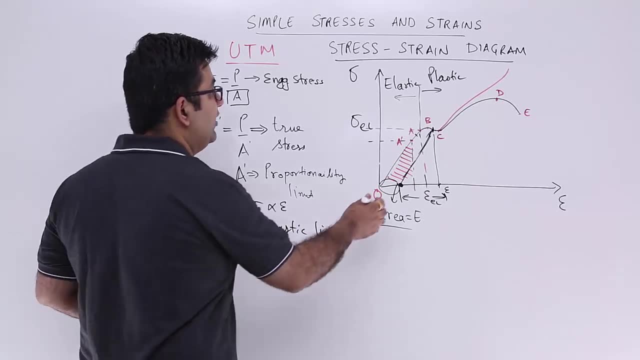 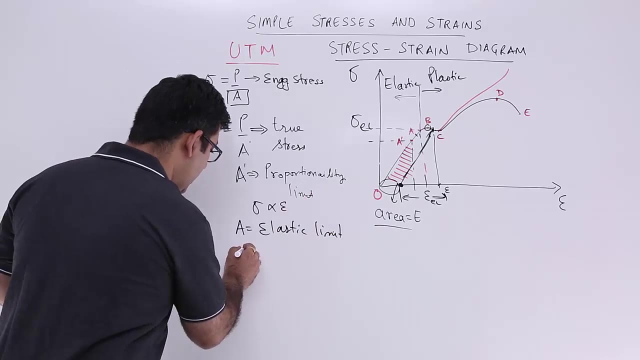 As The Permanent Deformation Actually Starts. You Can See The Material Is Getting Considerably Deformed, So This Is Where The Yielding This Is Called. 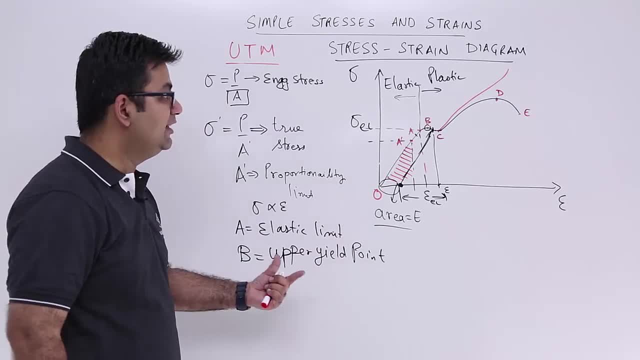 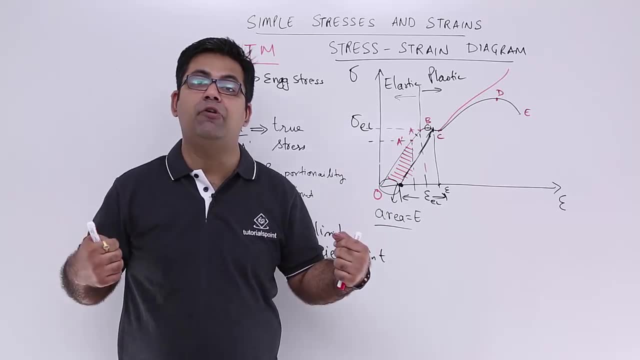 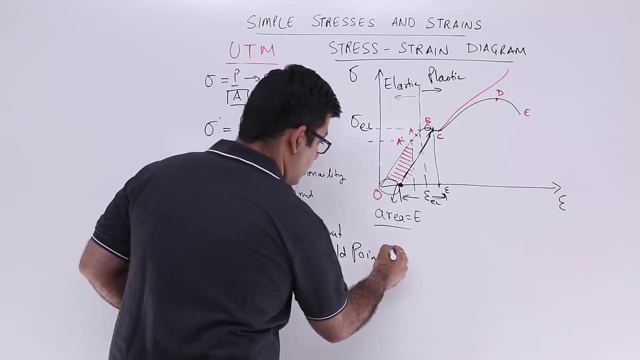 Yielding, That Is, Permanent Deformation, Setting In Formation Of The Flow Of The Material, You Know, During The Deformation Gets Started. So At This. 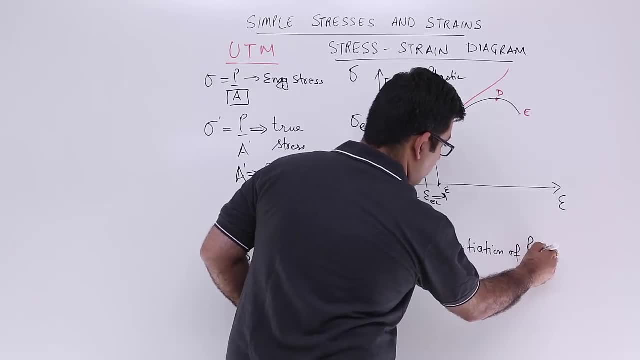 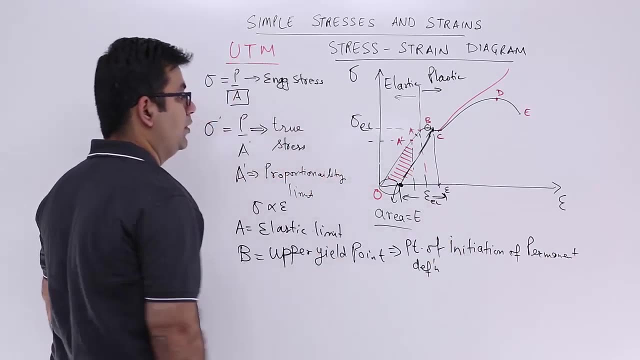 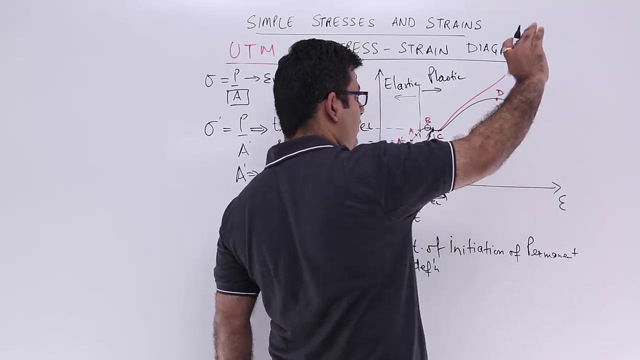 Point, The Permanent Deformation Is Initiated. This Is The Point Of Initiation Of Deformation. At Point C You Can See That There Is A. 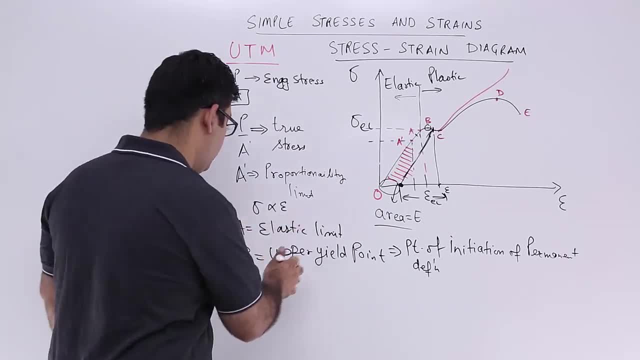 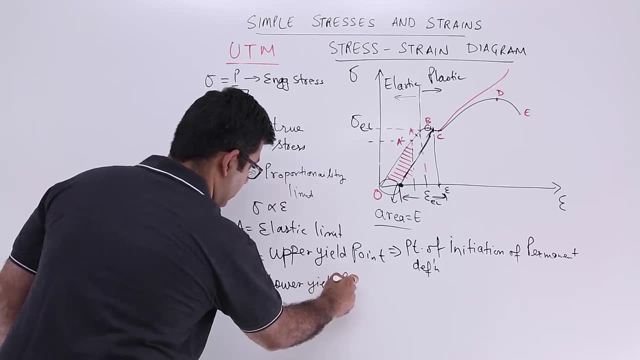 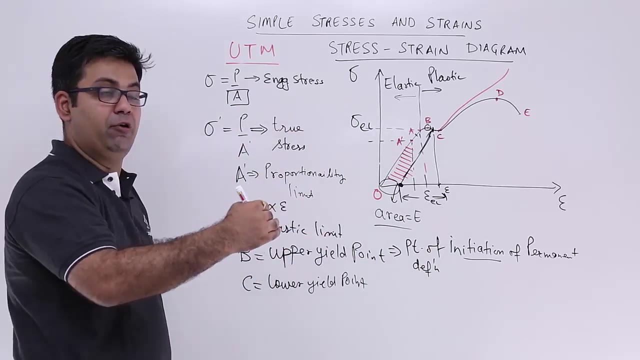 Sudden Increase In The Value Of Stress. So This Is Where Your Very Huge Permanent Deformation Of Very Important Thing Happens, At Or Beyond. 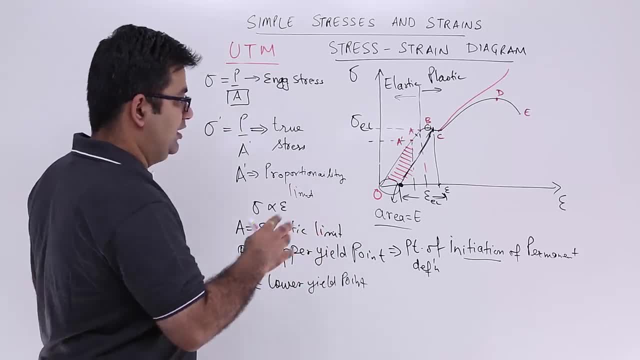 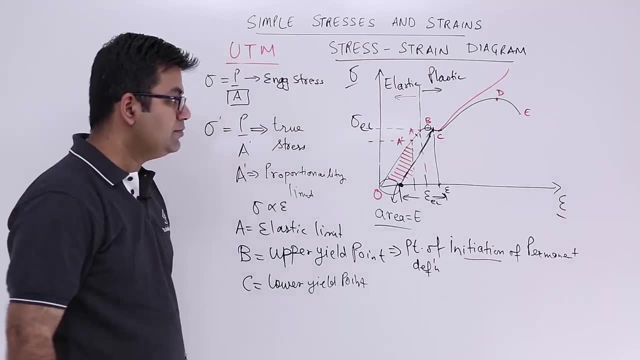 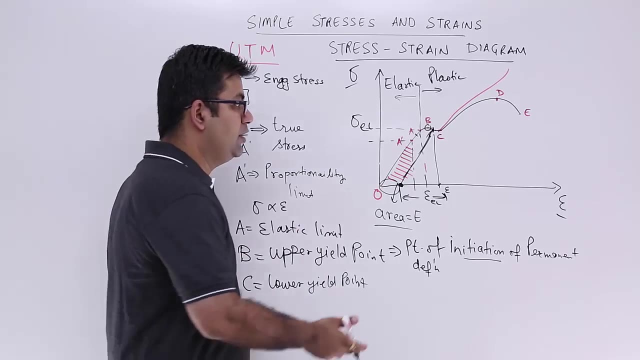 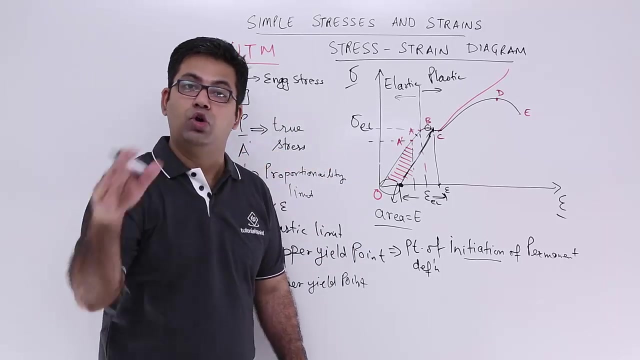 Point C, That Is The Lower Point. Okay, Now We Will Come To A Very Important Aspect Of This Particular Diagram. There Are You Apply. 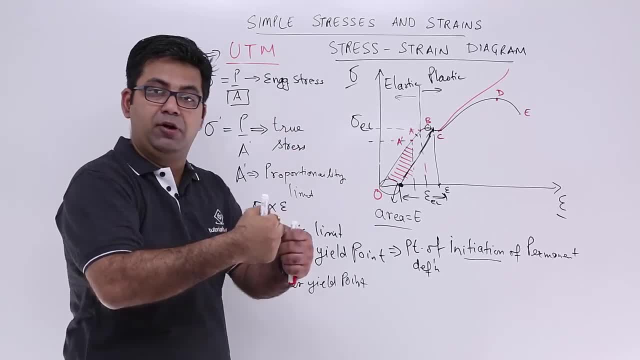 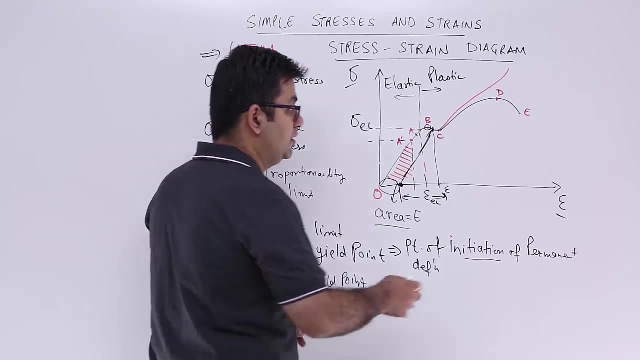 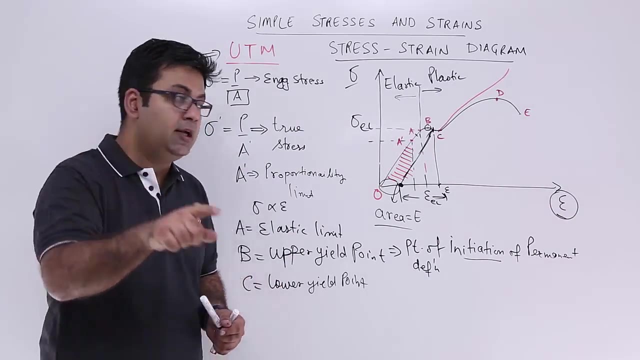 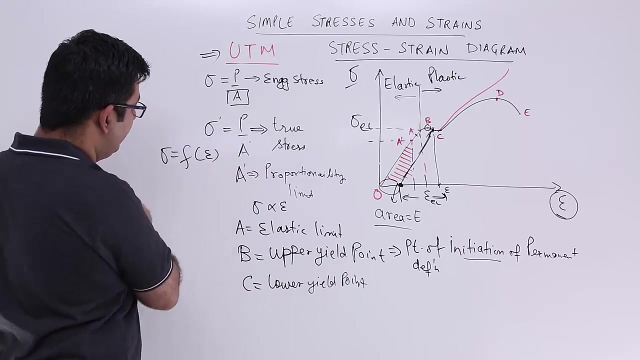 Load On To A Body, And That Is What You Are Doing In U T M. You Are Applying Either A Component And Side Load Or 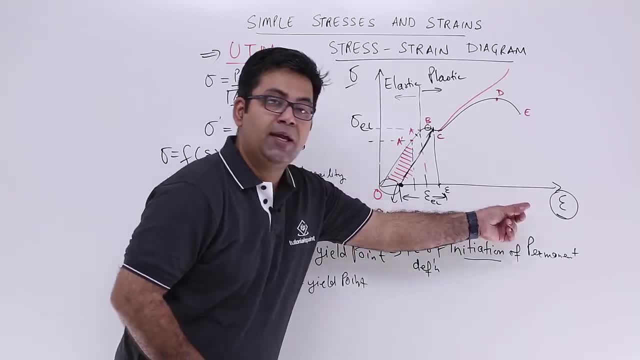 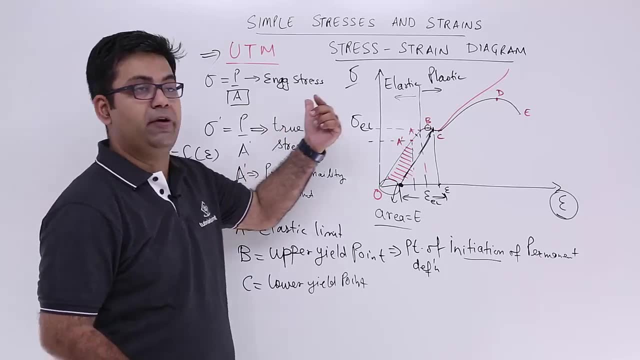 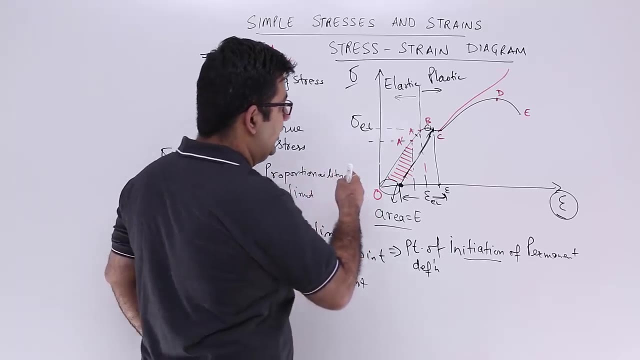 Compression. So In This, Sigma Becomes The Independent Variable, Sorry, Epsilon Becomes The Independent Variable And Sigma Becomes The Dependent Variable. So You: 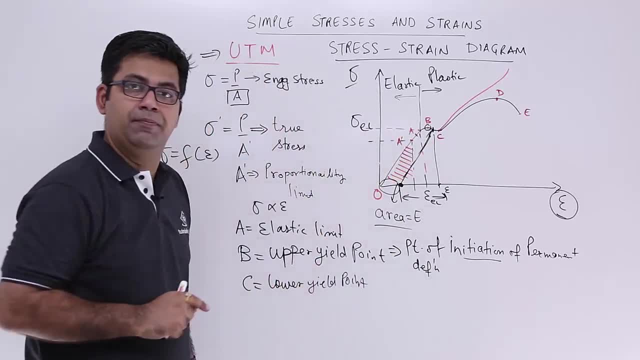 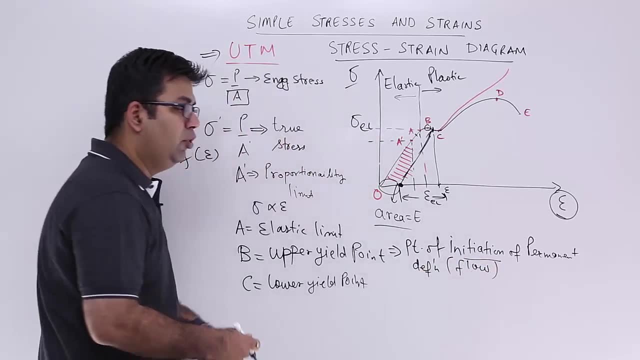 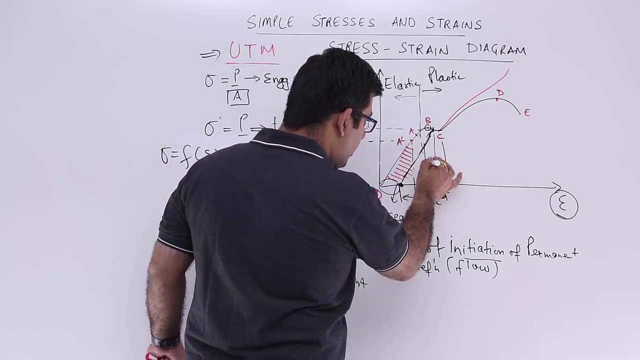 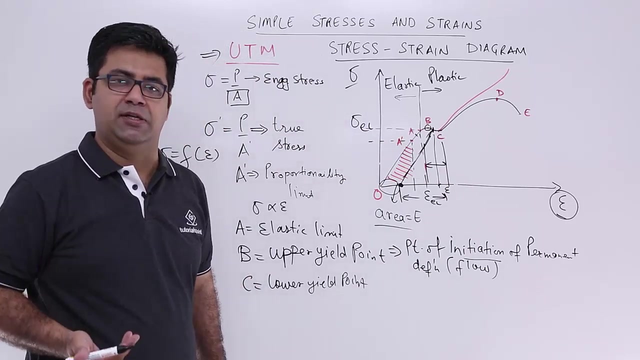 Can Have Can Now Understand It In Formation, That Is, The Material Starts To Flow Like A Fluid, It Starts To Get Deformed, Very, Very. 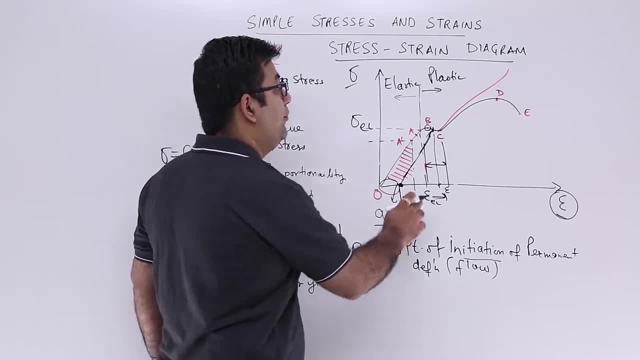 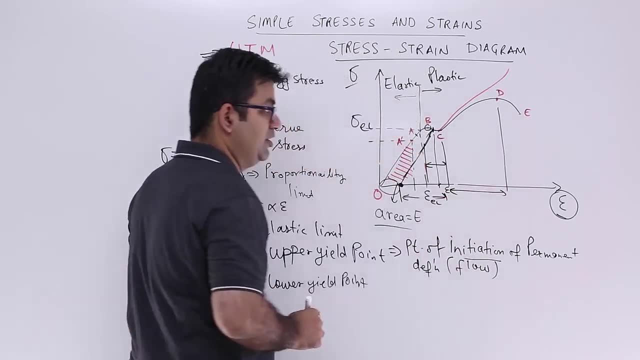 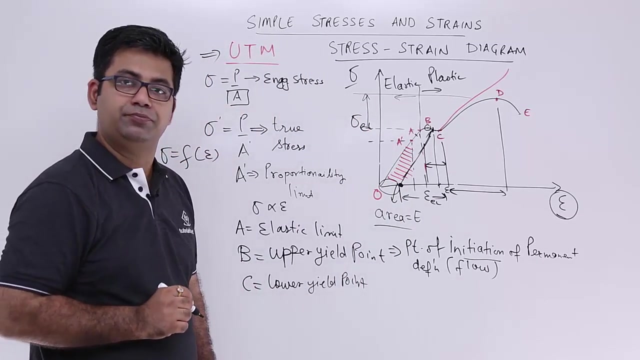 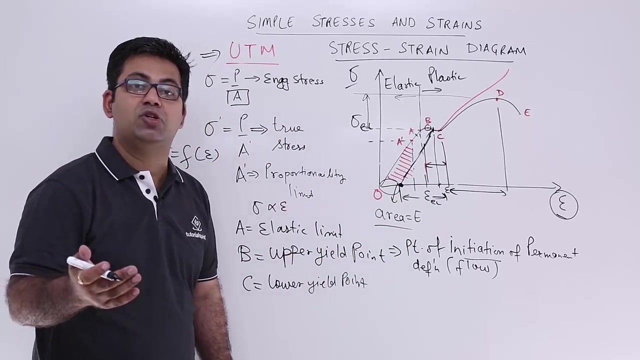 Considerably So To Resist This Much Amount Of Deformation The Material There Is A Very High Value Of Increase In The Value Of Stress. Okay. 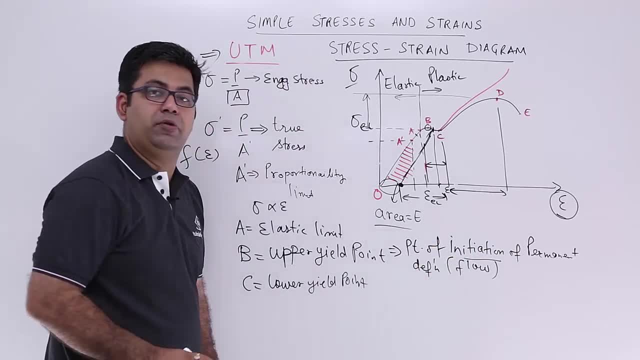 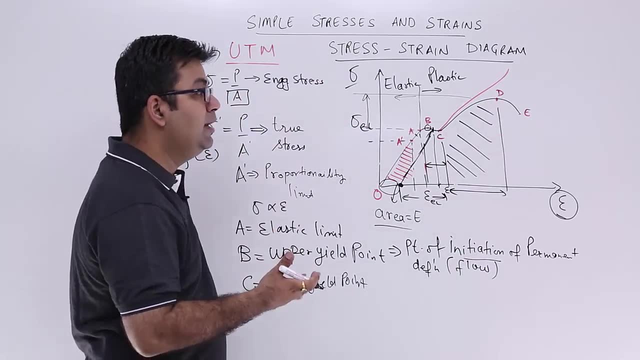 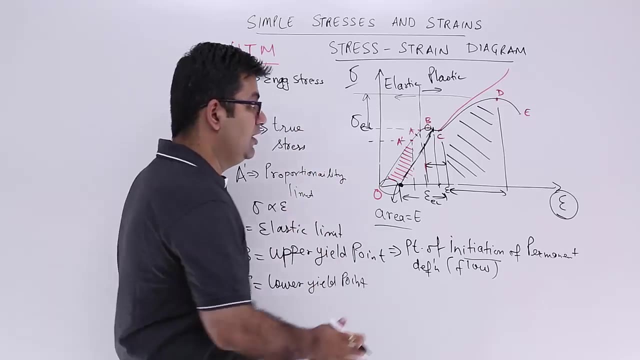 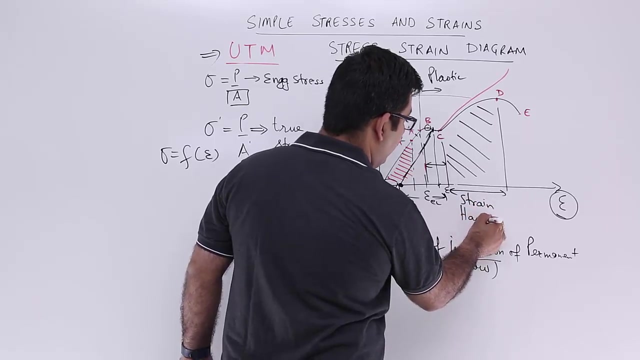 This Means That The Resistance Provided By The Material Has Gone Considerably High To Resist A Of Stress In The Body. So This Region Is 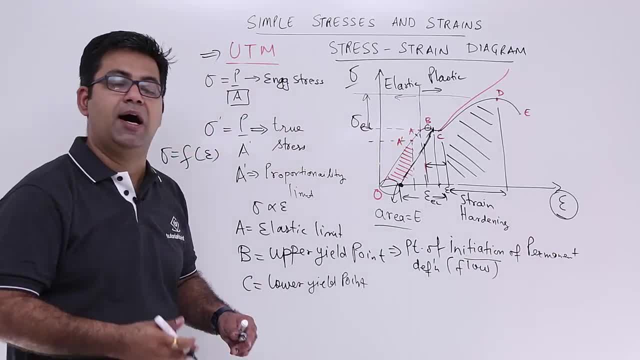 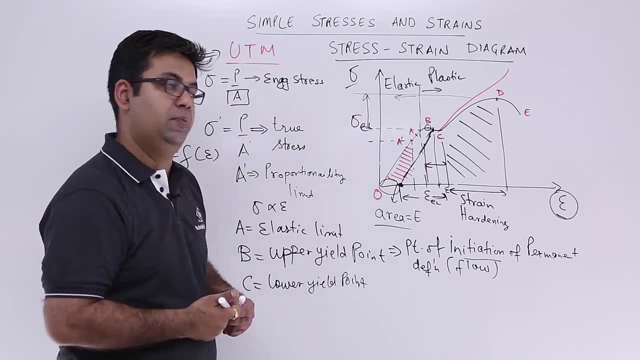 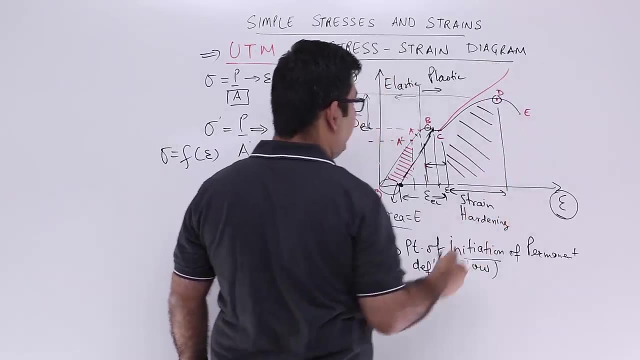 Called Strain Hardening. Strain Hardening, Which Means That The Material Now Starts To Behave Like A Hard Material Due To The Maximum Stress. 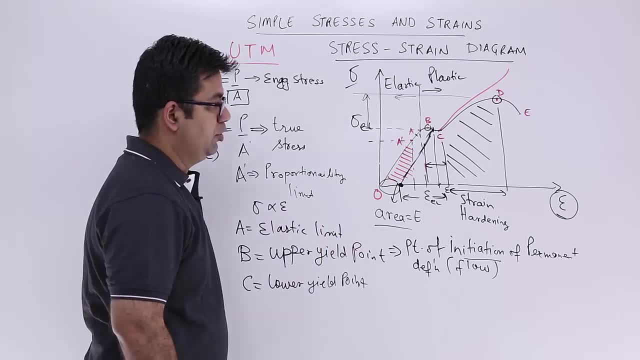 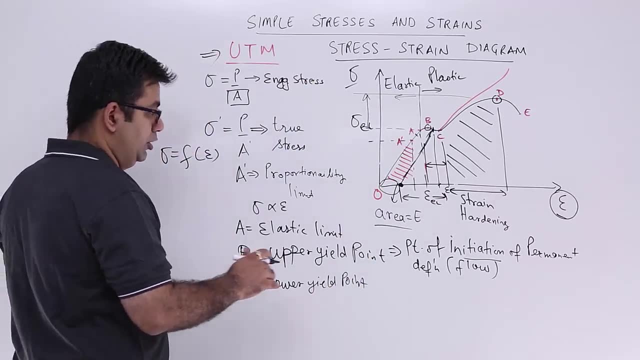 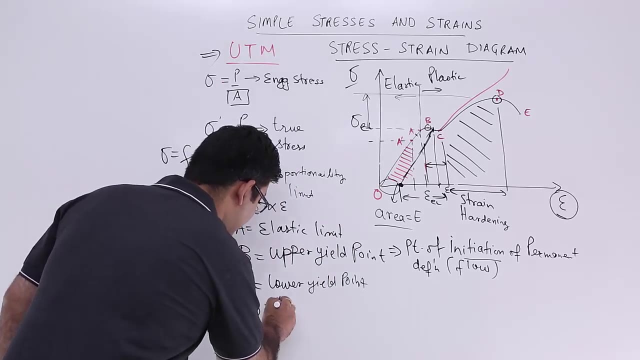 That The Body Can Produce To Counter The Elongation Or The Deformation. This Means This Is The Ultimate Stress Which Can Be Produced In. 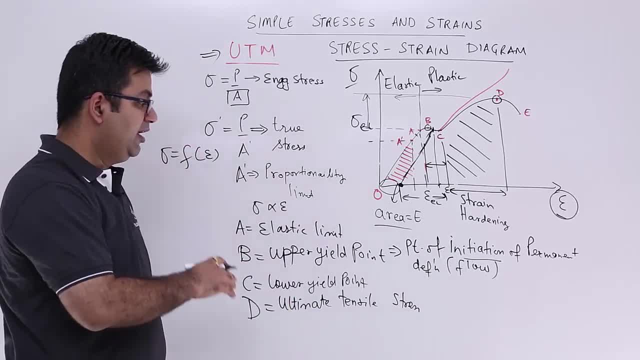 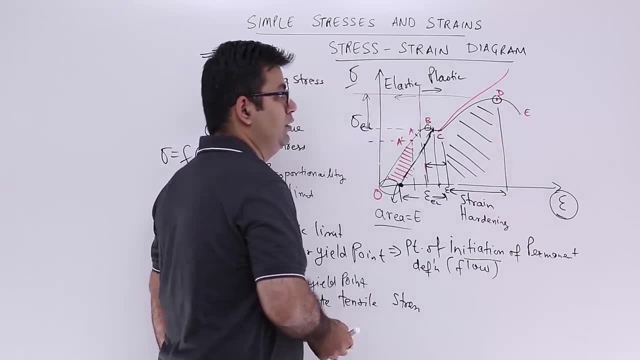 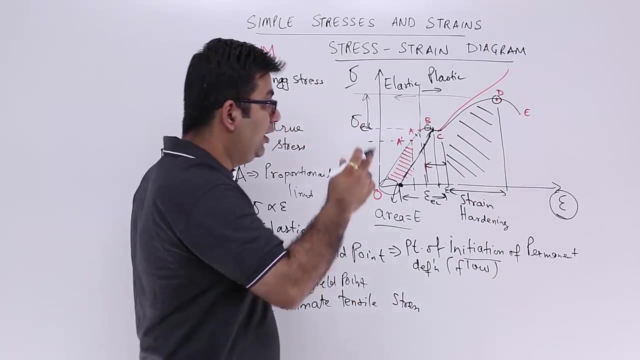 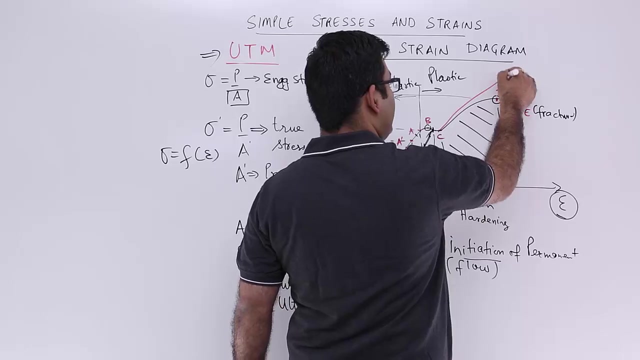 The Body. Now You Cannot Have, You Know, A Stress Value Which Is More Than This. Now Why There Is A Dip In This Particular. 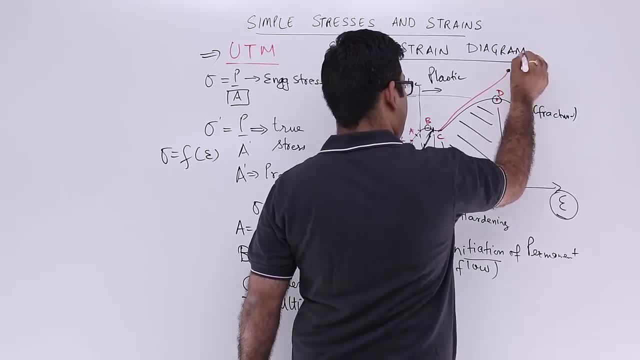 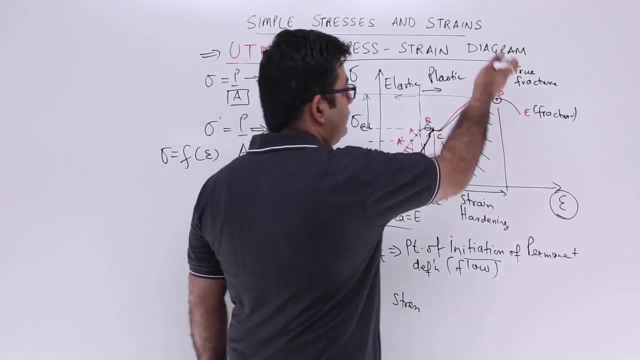 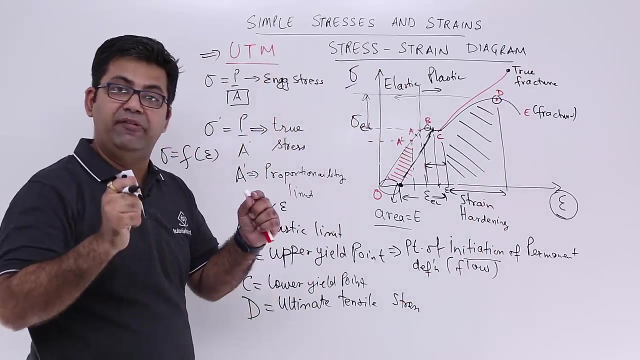 Of Beyond Point E And Why, Or Corresponding To True Stress, Why The True Stress Keeps On Going, Or The True Fracture Point Is: 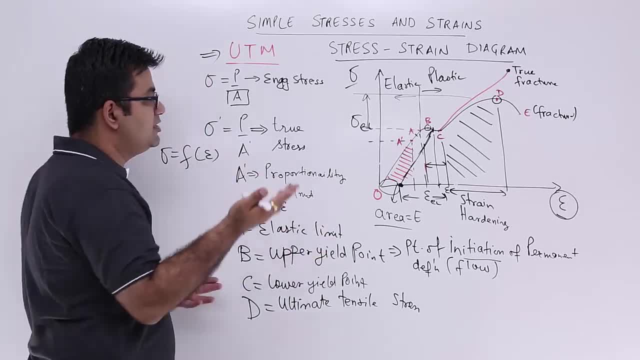 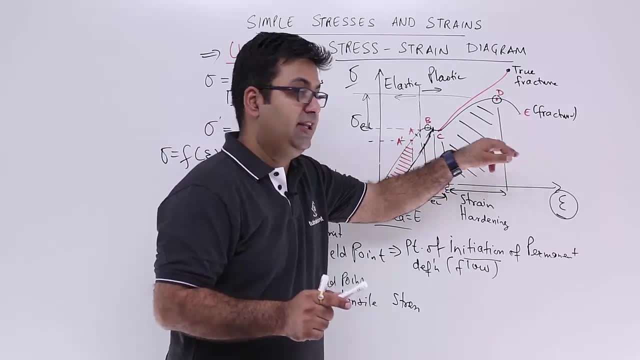 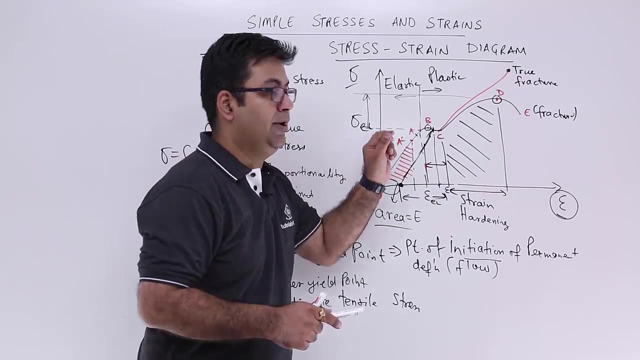 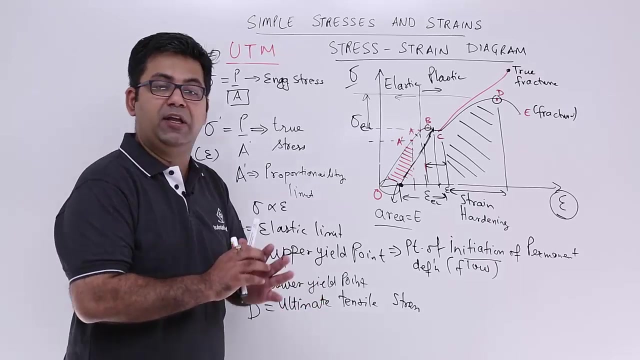 At A Higher Value Of Stress As Compared To The Engineering. Is That Okay? Your Area Is Constantly Decreasing. At Point D You Cannot Have 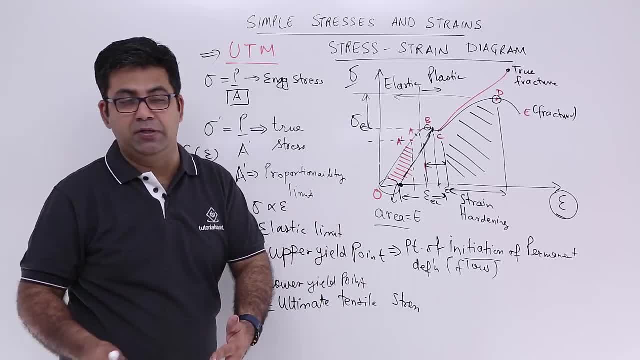 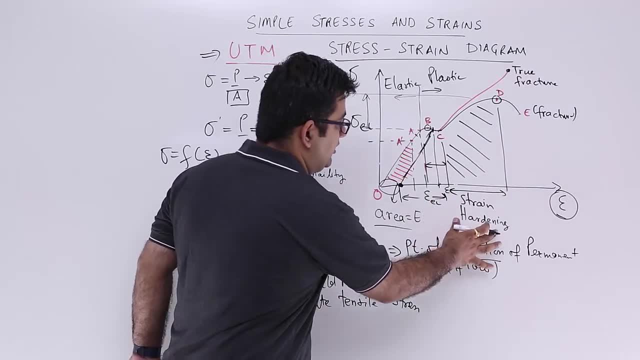 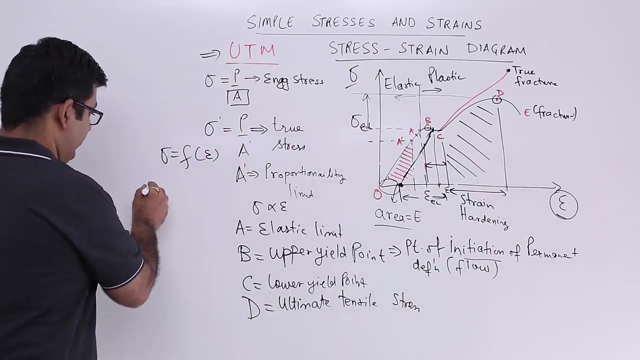 The Resistance By The Material Higher Than Point D. So Now Your Material Will Not Be A Phenomena Occurs, Which Is Called Necking, Which 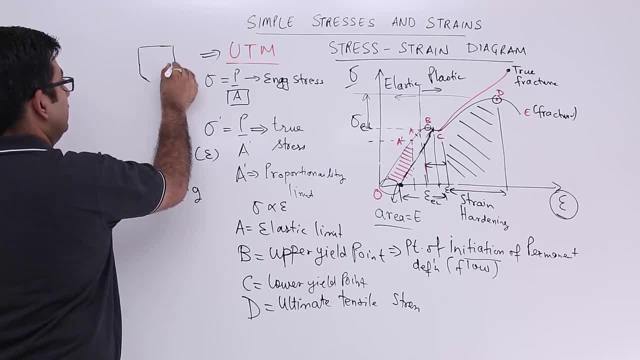 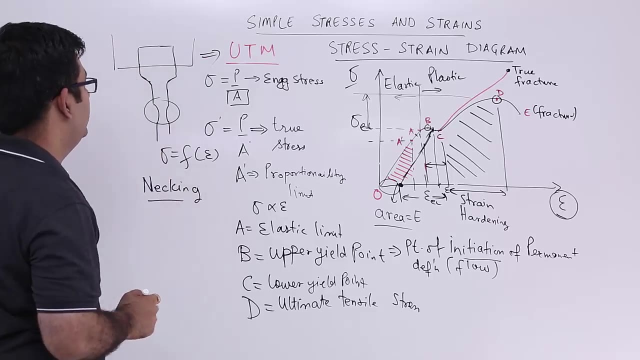 Is Called Necking, That Is, If This Is The Specimen. If This Is The Specimen, Okay, You Have A Neck Parts To Produce Of. 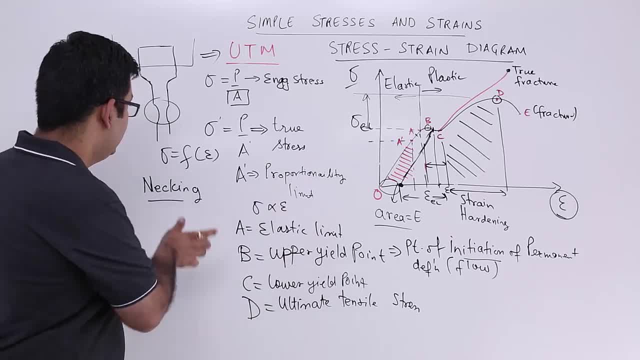 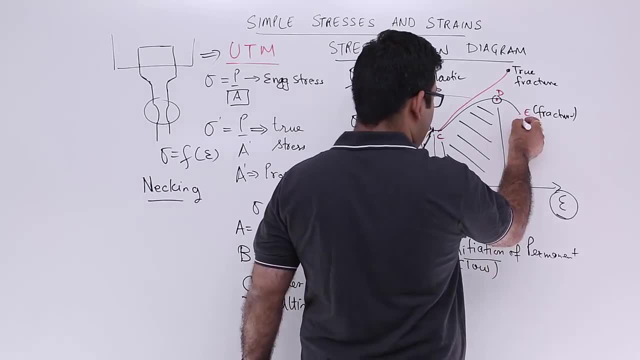 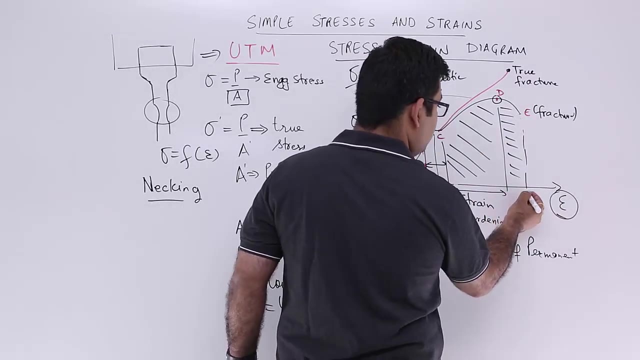 Get Formed At Point D And You Keep On Stretching It, You Keep On Stretching It. This Will Keep On Getting Thinner, Okay, But 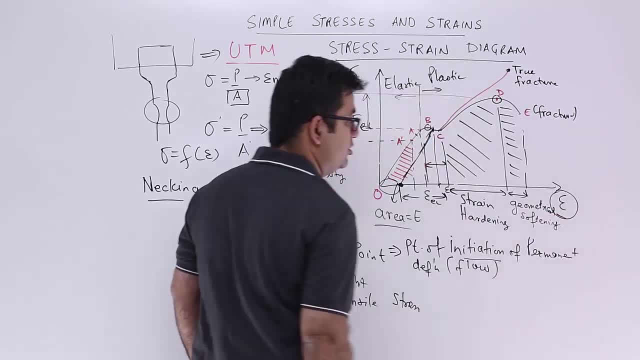 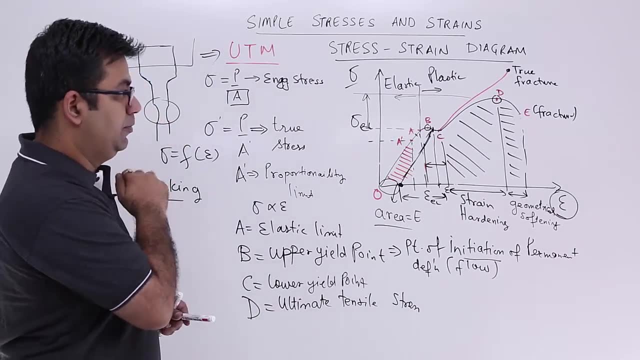 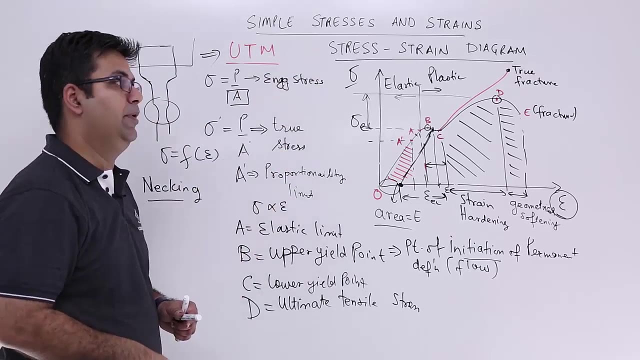 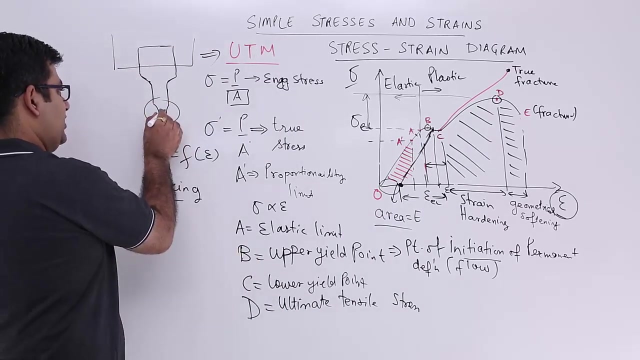 Why Geometrical Softening Your Material Has Started To Become A Behave As A Soft Material. All Right, Now Let's Talk About That Dip. 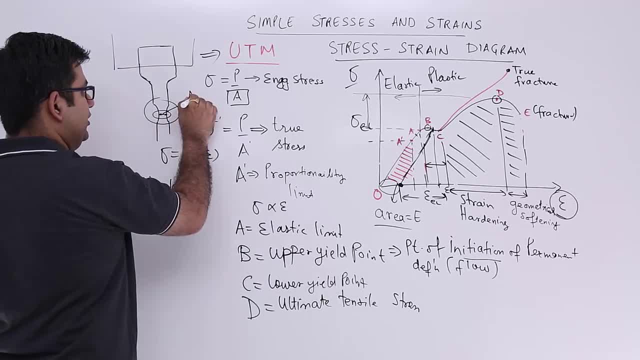 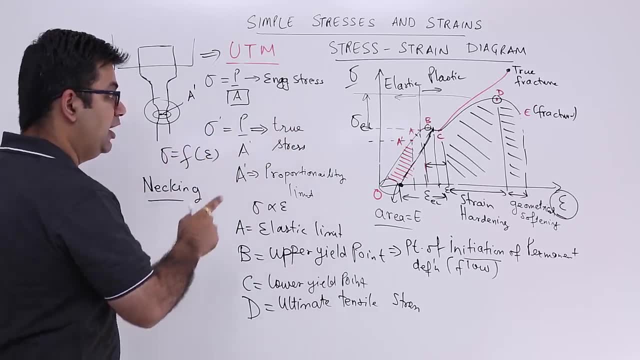 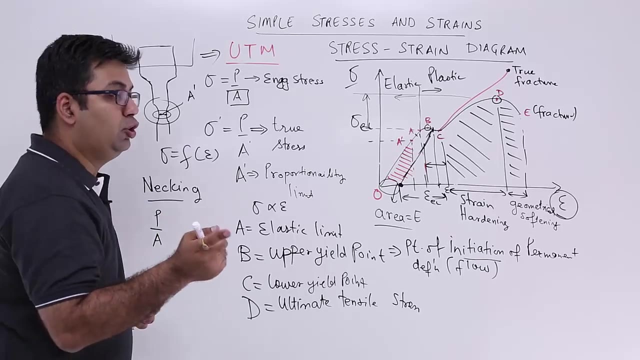 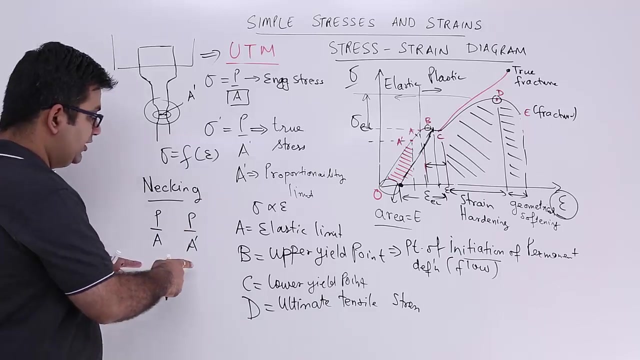 Over There And Why That The Original Area Is A. So At The Point D The Engineering Stress Value Is P By A. But The True. 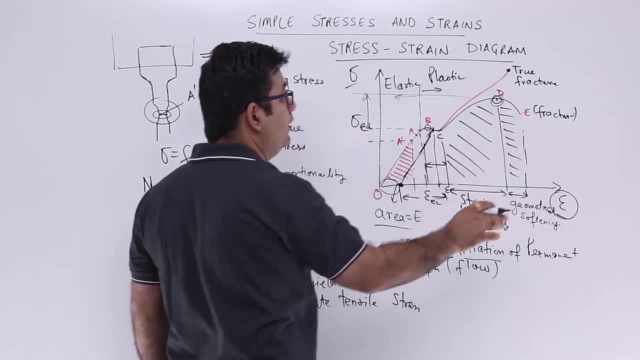 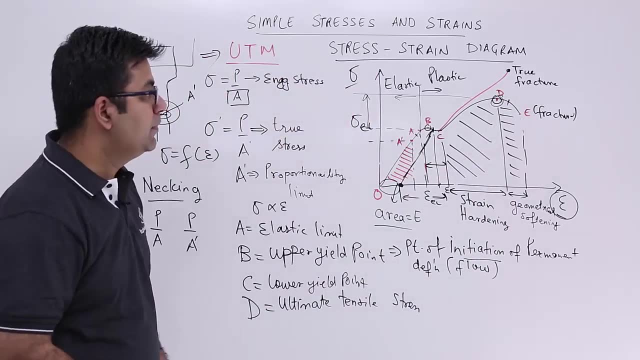 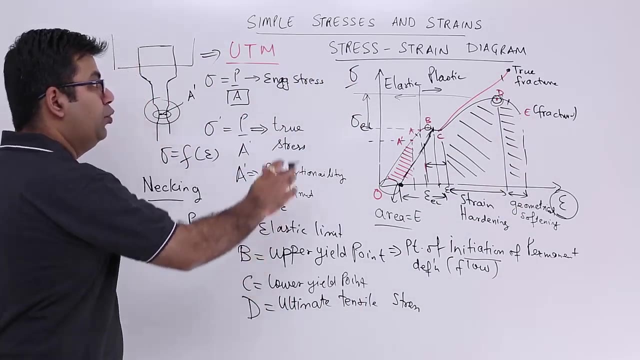 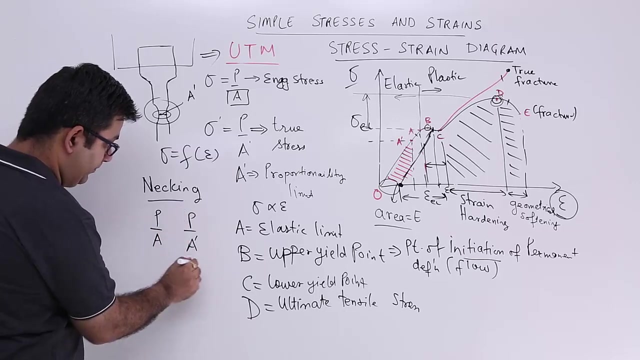 Stress Value Is P? Upon A Dash. Now This Point Beyond Point D. So Beyond Point D On The Engineering Graph. And Let Us Say You: 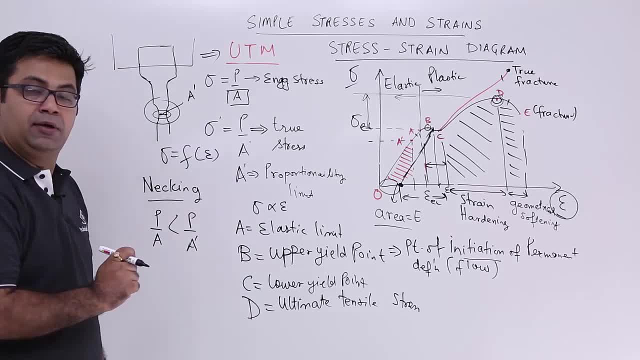 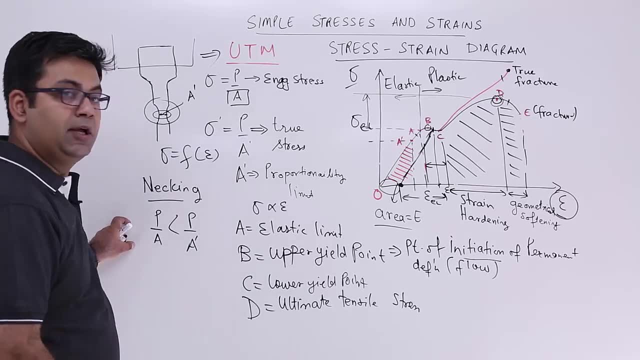 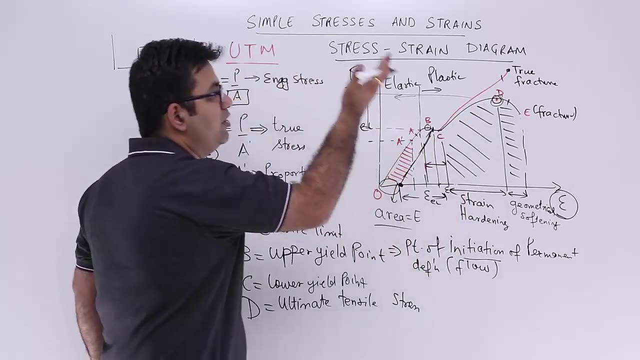 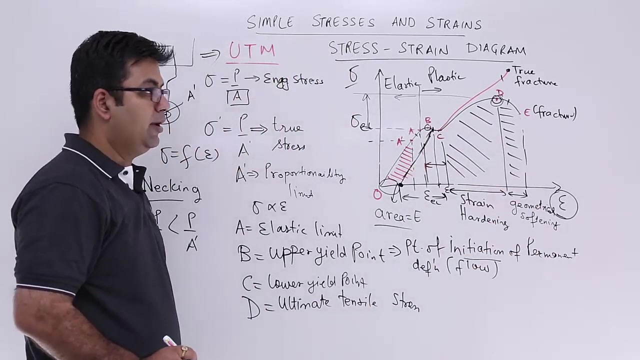 Have A Corresponding Point On The True Graph Both In Both Presses, Compared To The Stress. So In A General Sense The Stress In The 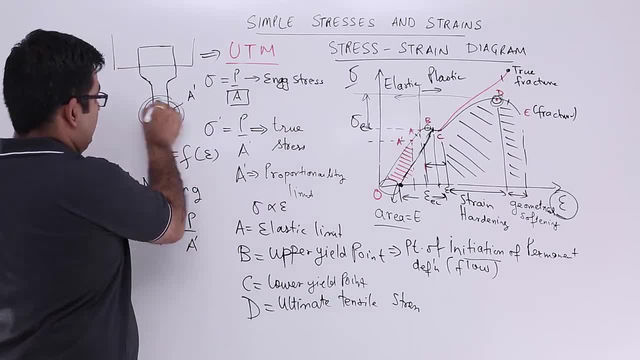 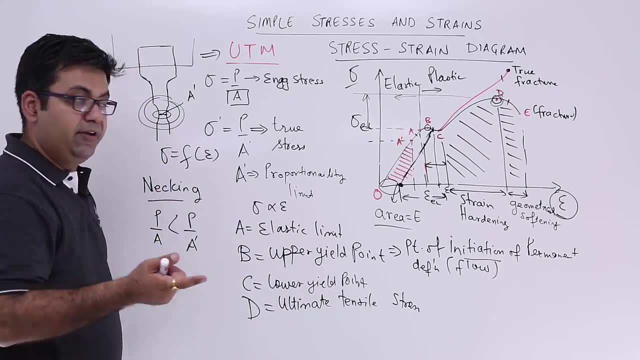 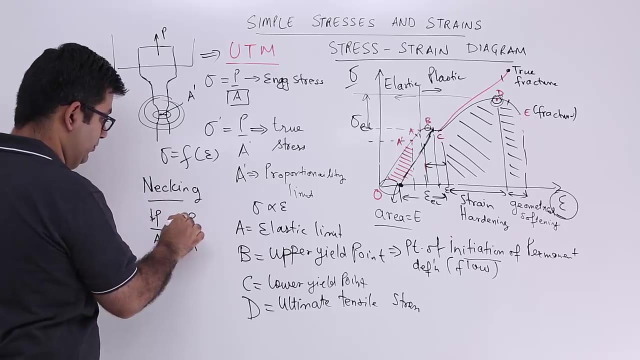 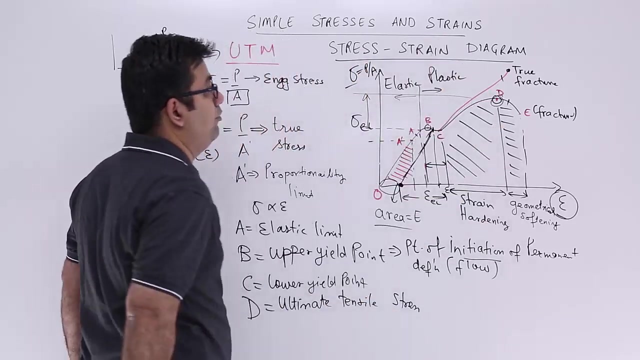 True Graph Will Always Go Up. Okay, Okay, Accepted, But Again The Question Is, Why This Specimen? So We Start Reducing The Load, We Start. 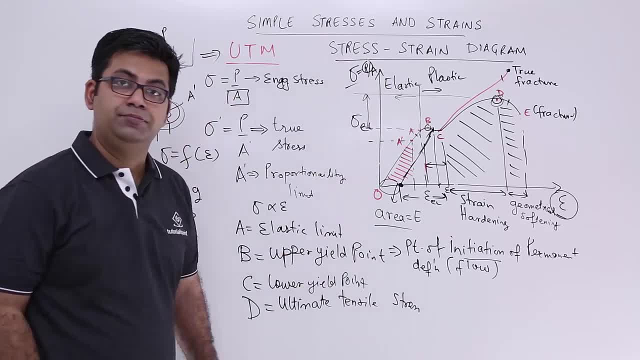 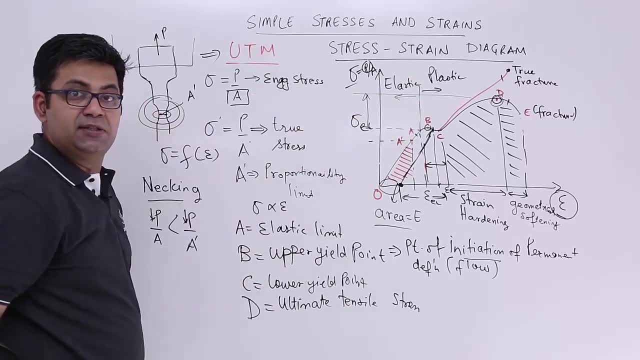 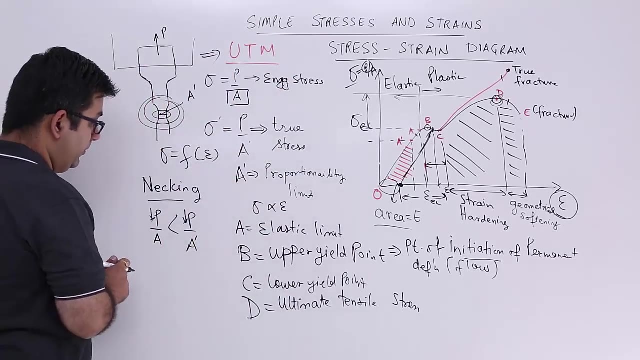 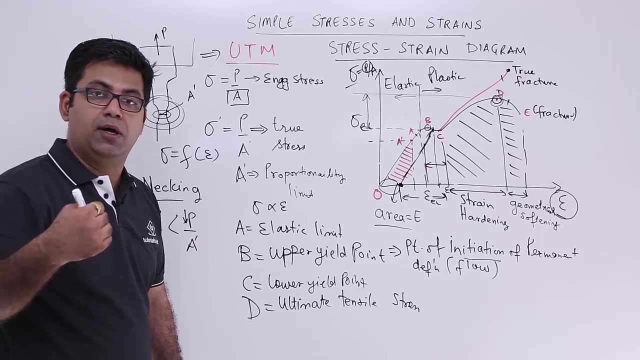 Reducing The Load. If You Look At Sigma Over Here, This Is A Direct Formula Which Is P By Increasing The Load. Okay, But Still. 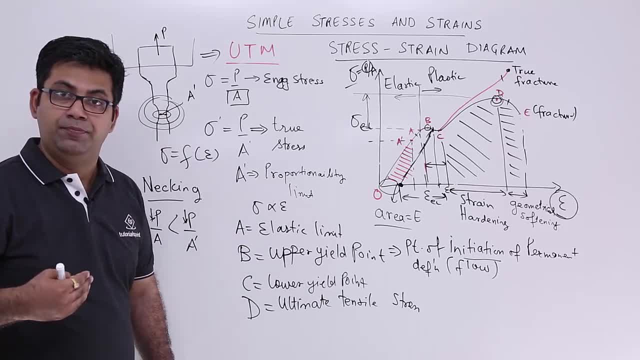 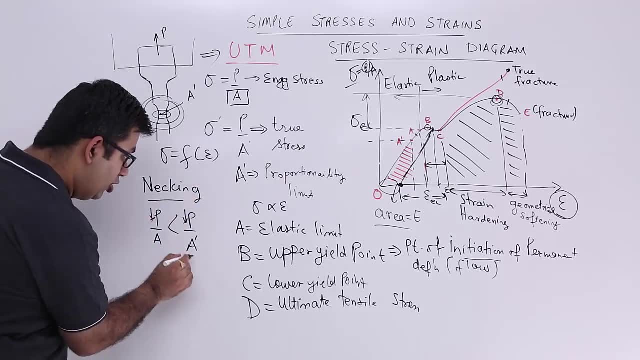 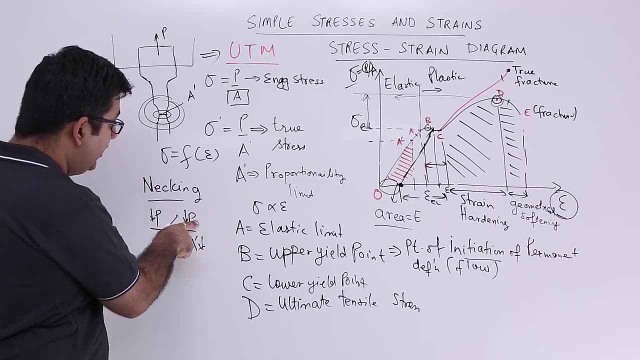 You Are Applying The Load, You Are Not. You Know. Your Increment In The Load Has Reduced. Increment In The Load Has Reduced To This One. 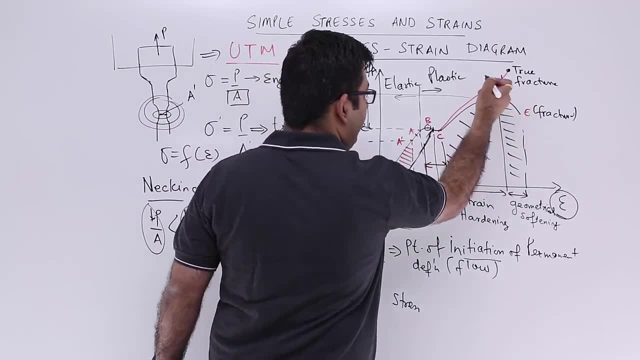 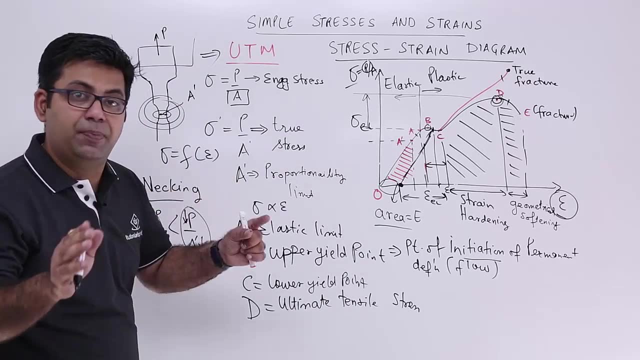 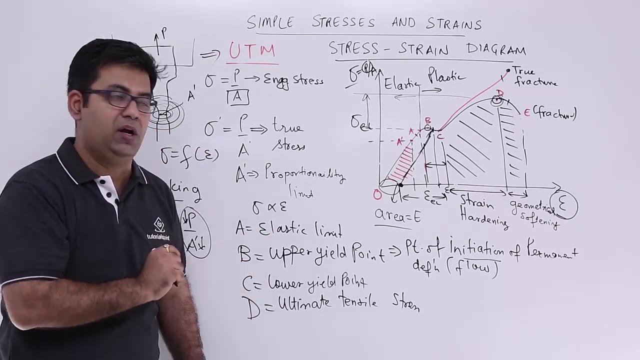 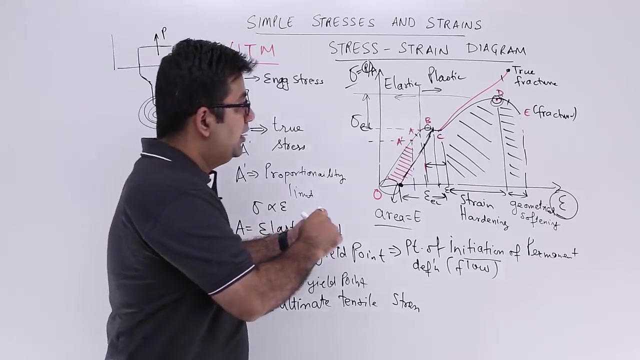 So This Stress Will Still Be Higher As Compared To This. So There, That Is Why There Is A Dip Over Here And It Fractures. 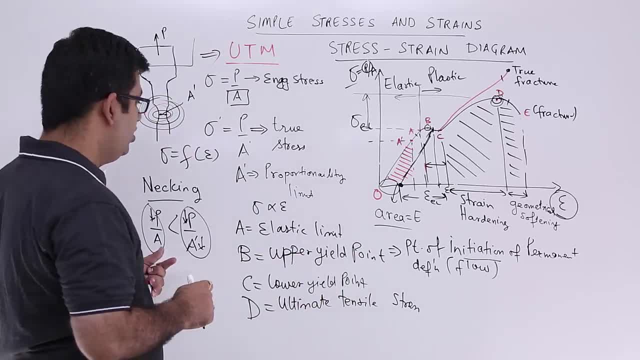 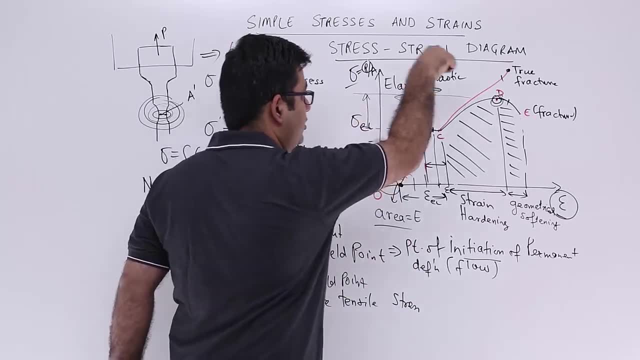 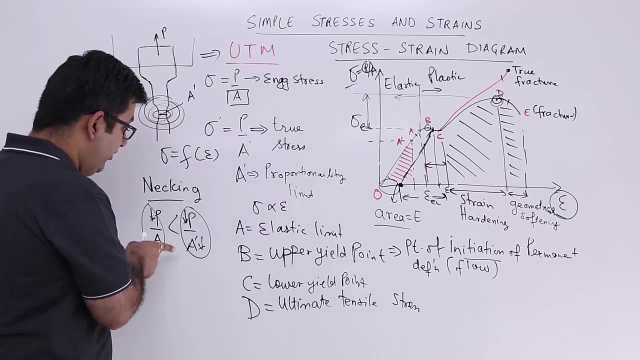 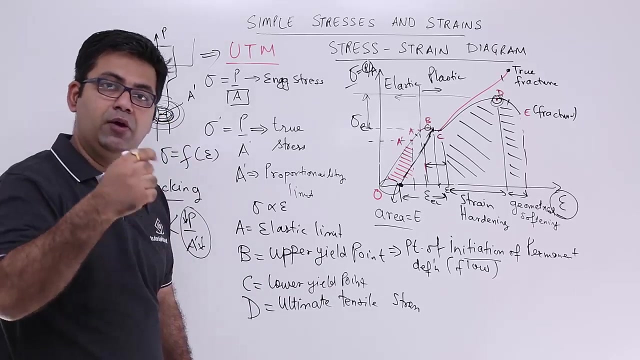 At The Body. So What We Do, We Are Reducing The Load. So When You Reduce The Load, This Sigma Is P By. So If 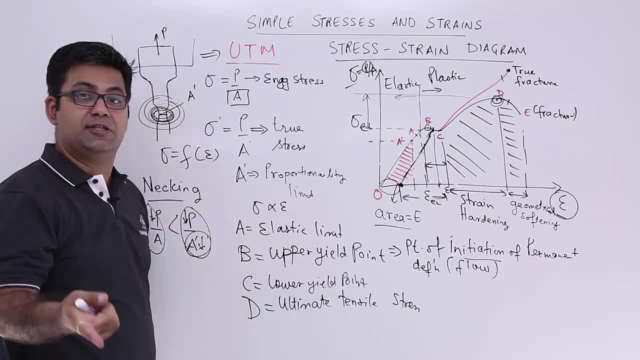 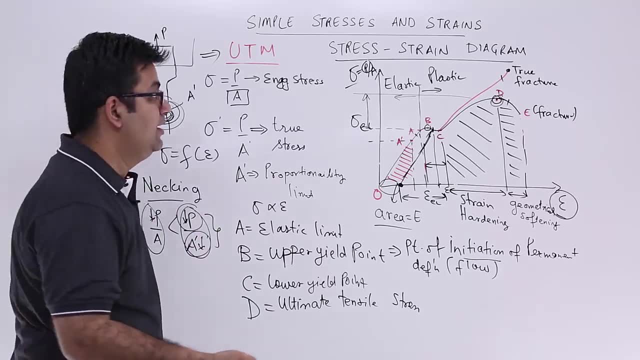 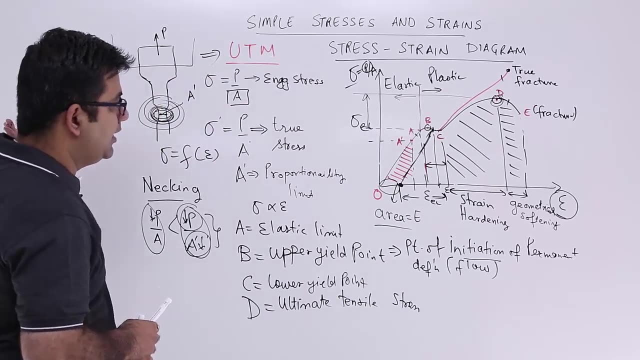 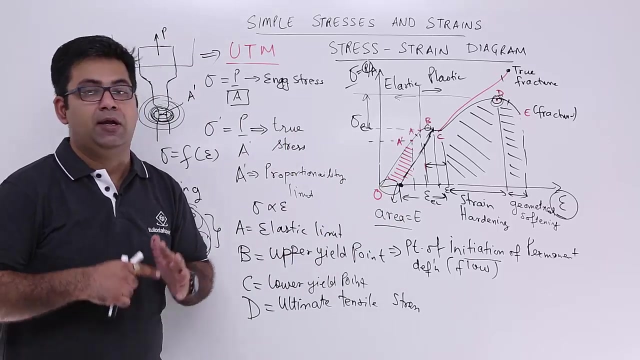 P Reduces, Sigma Has To The Reduction In The Load, So This Stress Is Still Higher As Compared To The Stress In The Engineering Graph.